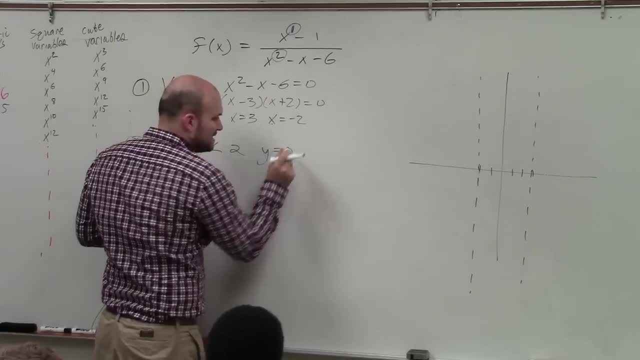 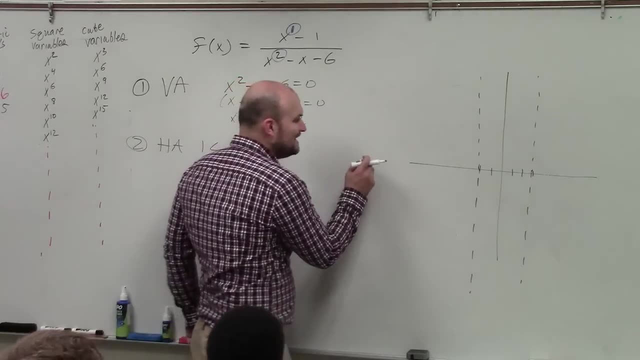 asymptote of y equals 0.. Not 0,, but make sure it's y equals 0,, because what that needs to tell you? if x equals produces a vertical line, y equals is going to produce a horizontal line. Is everybody following me so far on my graph? 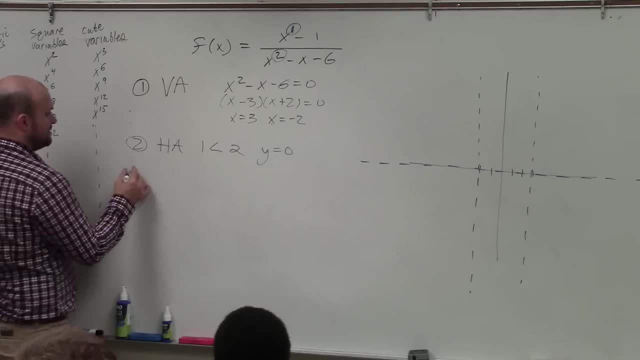 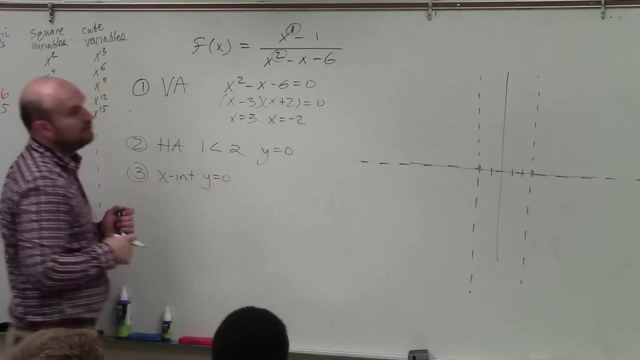 Next thing is determining the x and the y intercepts. I showed you guys that little example over there. The x intercept is when y is equal to 0.. Well, obviously, ladies and gentlemen, we're talking about a function here, so we don't. 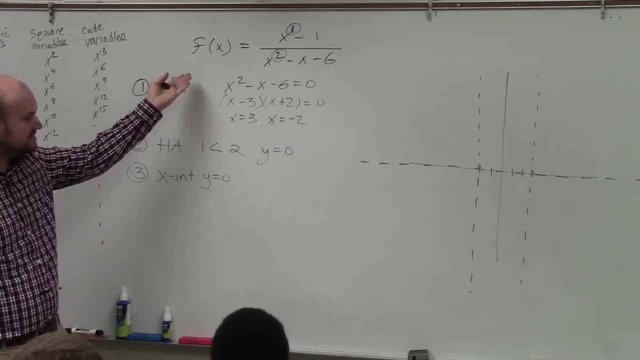 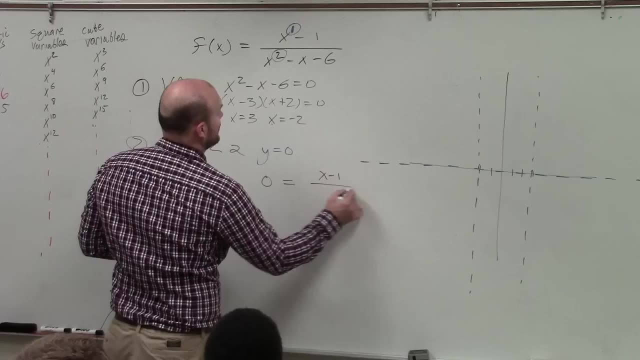 have a y, we have an f of x, But the same process applies. You're going to replace f of x with 0 and then solve for x. 0 equals x minus 1, all over x squared minus x minus 6.. 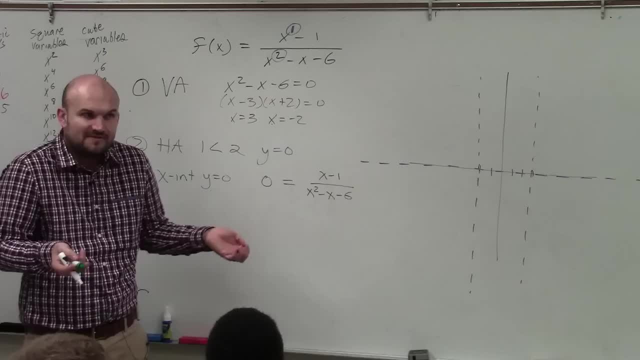 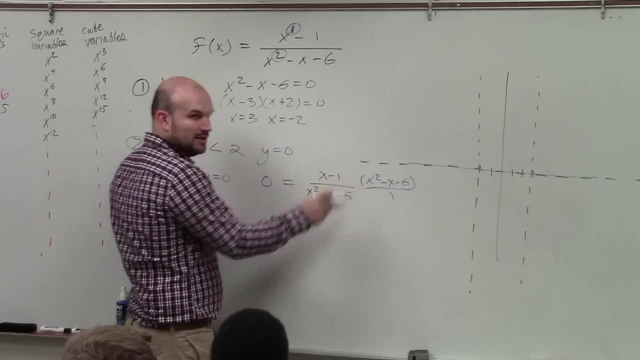 Well, whenever you have a variable in the denominator, we've got to get the variable off the denominator. So I can do that by multiplying. I can do that by multiplying by its reciprocal. I'm not going to multiply by the total reciprocal. like, totally flip that over, because then 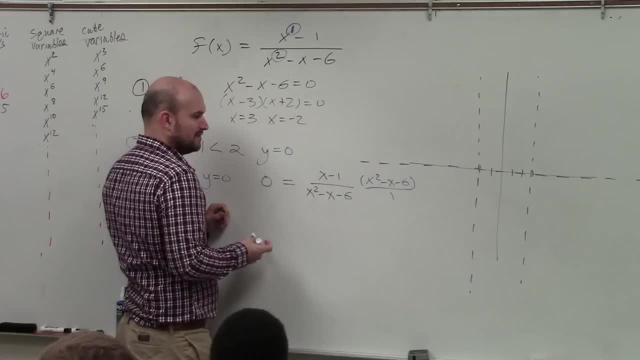 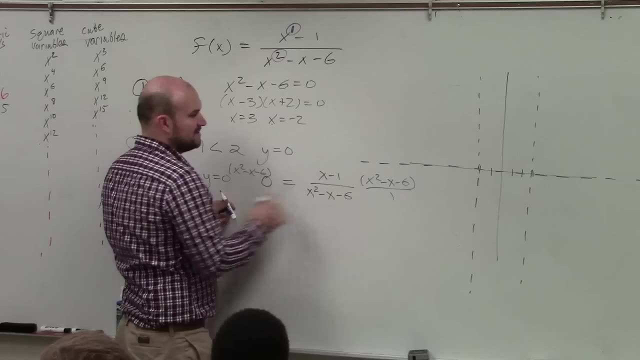 I'd still have an x minus 1 in this denominator, or it's not going to help me out over there. So I'm just going to multiply by this to get this off the denominator, and then I multiply it over here, And what happens? 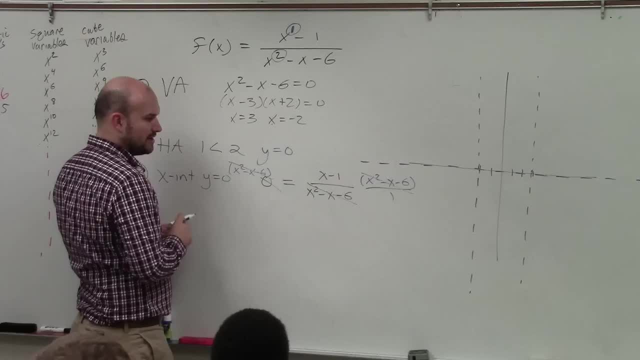 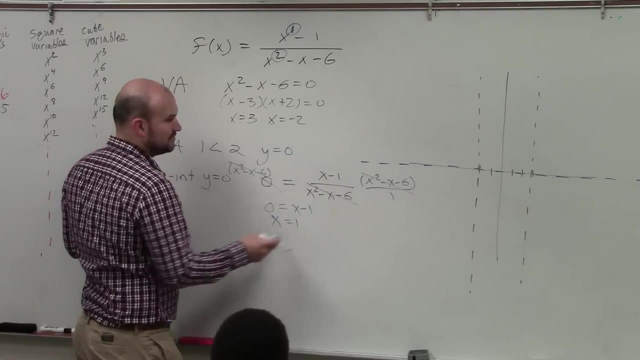 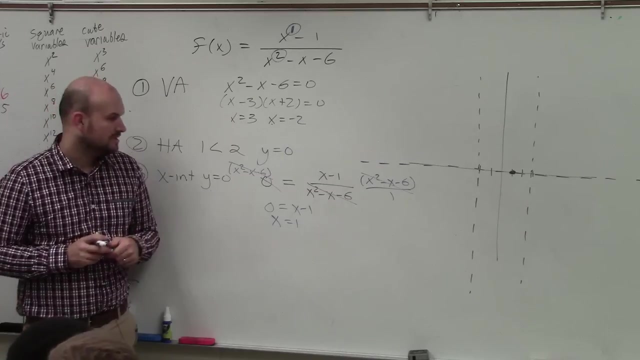 That divides to 1. This goes to 0. So I'm left with 0 equals x minus 1.. So therefore my x intercept is: x equals positive 1.. Right, Make a nice big point. OK, That's an ad. 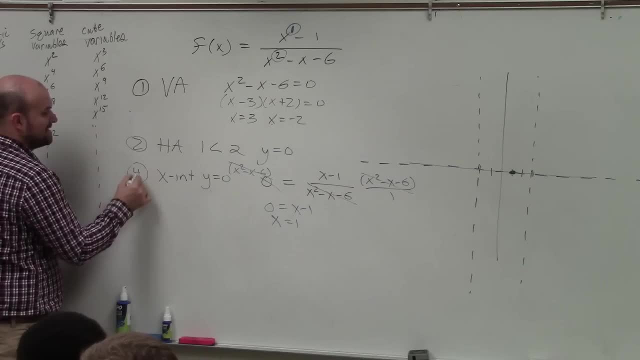 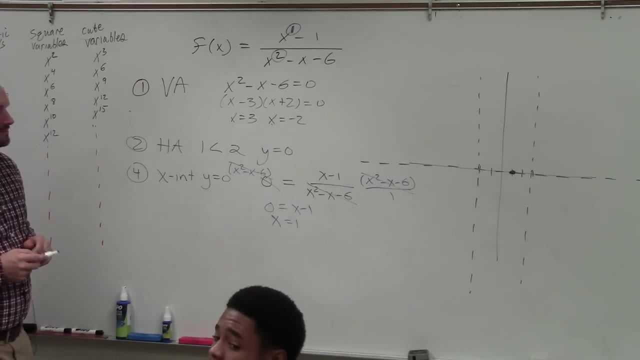 oh, I'm sorry I skipped number 3: slant asymptotes. We don't have slant asymptotes in this case. Step number 5.. Wait, wait, wait on step 4, why do you multiply by the reciprocal if it's just over 1?? 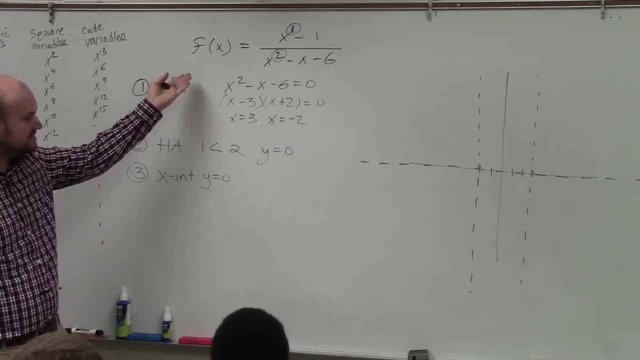 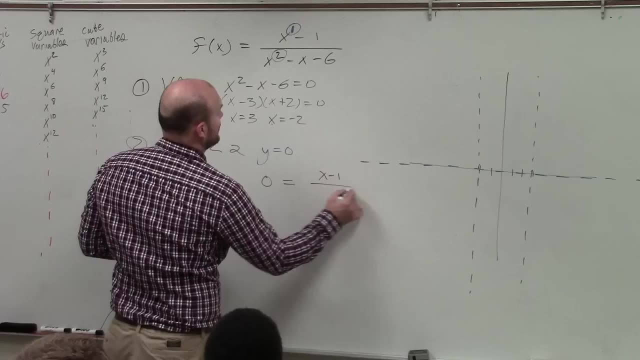 have a y, we have an f of x, But the same process applies. You're going to replace f of x with 0 and then solve for x. 0 equals x minus 1, all over x squared minus x minus 6.. 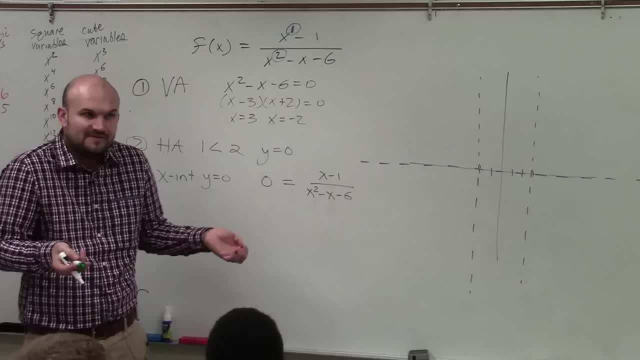 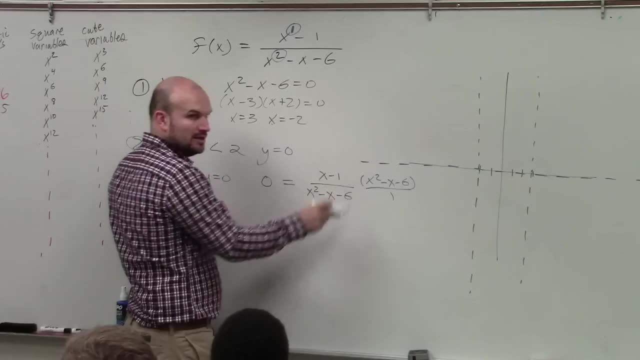 Well, whenever you have a variable in the denominator, we've got to get the variable off the denominator. So I can do that by multiplying by its reciprocal. I'm not going to multiply by the total reciprocal. like, totally flip that over, because then 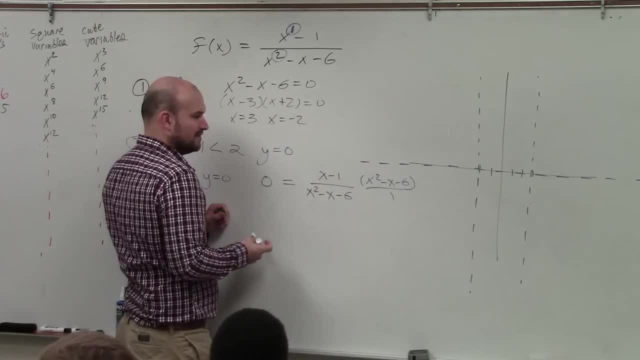 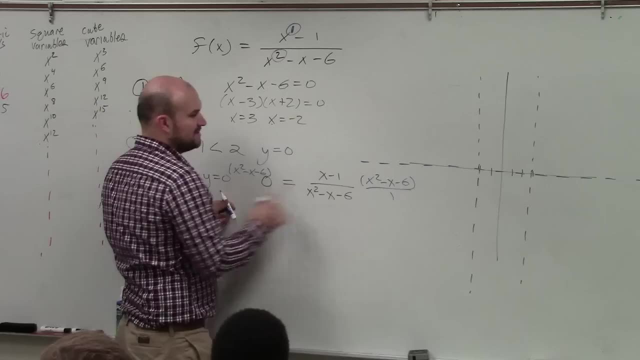 I'd still have an x minus 1 in this denominator, or it's not going to help me out over there. So I'm just going to multiply by this to get this off the denominator, and then I multiply it over here, And what happens? 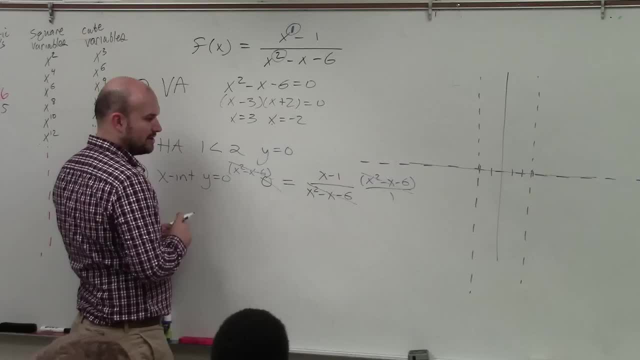 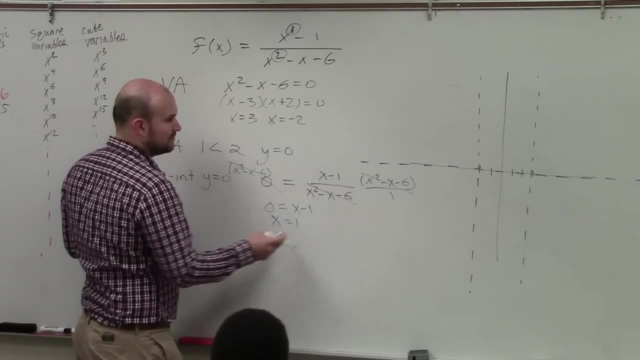 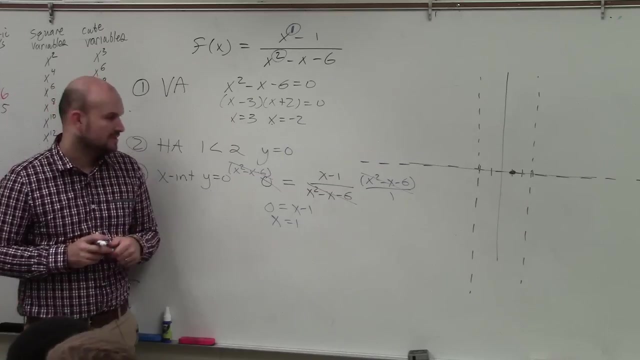 That divides to 1. This goes to 0. So I'm left with 0 equals x minus 1.. So therefore my x intercept is: x equals positive 1.. Make a nice big point, OK? Oh, I'm sorry. 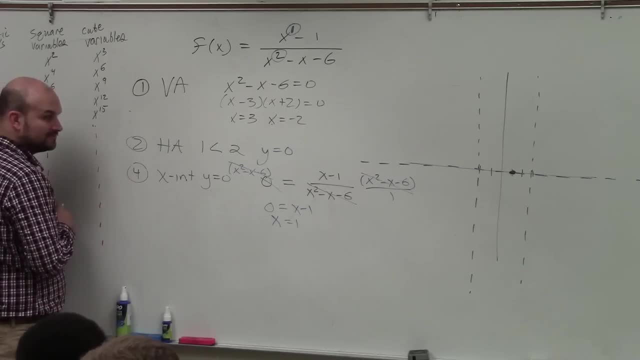 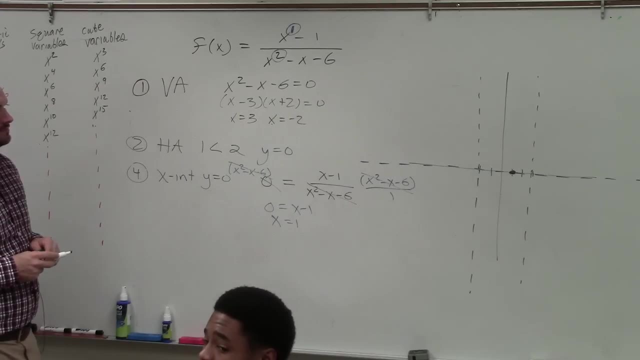 I skipped number 3, slant asymptotes. We don't have slant asymptotes in this case. Step number 5.. Wait, wait, wait, On step 4, y equals. Well, I just want to get rid of what's in my denominator. 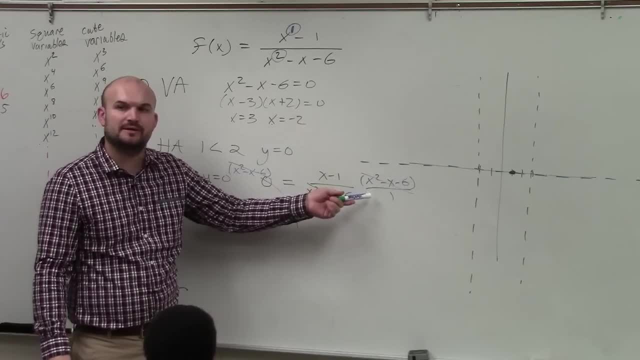 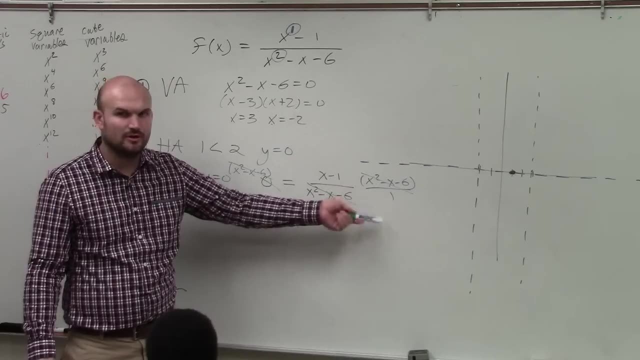 So I'm multiplying by the reciprocal of that. That eliminates what's in that denominator, Right? If you multiply by the reciprocal, then you have an x minus 1 in the denominator. You don't want to have any variables in the denominator. 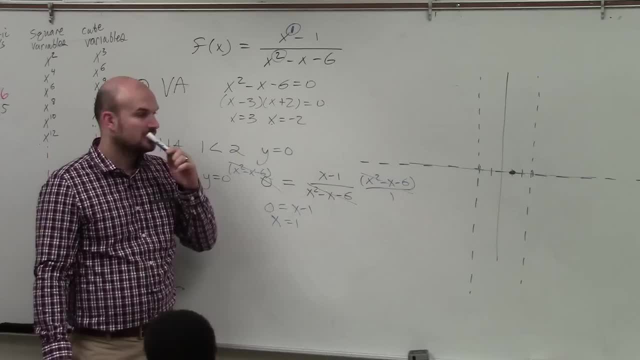 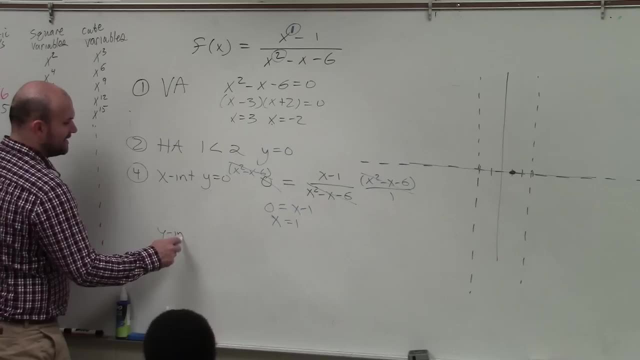 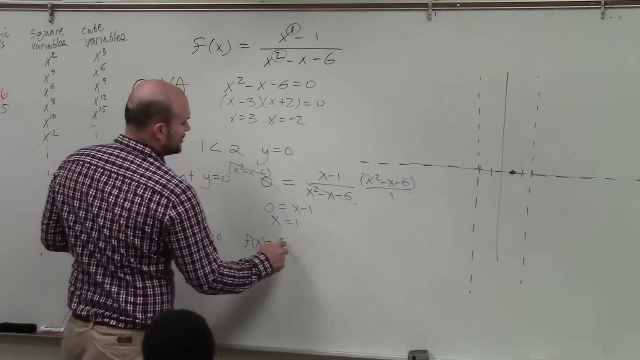 So I'm just multiplying by what's in the denominator. OK, OK. So now the step. next one is to find the y, What's the y-intercept. y-intercept x equals 0.. So in this case I have f of x equals 0 minus 1, divided by 0 squared minus 0 minus 6,. 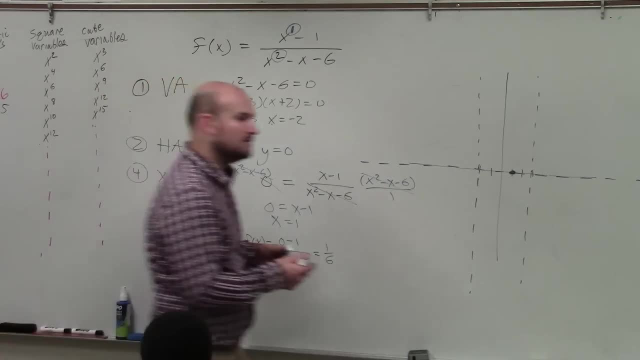 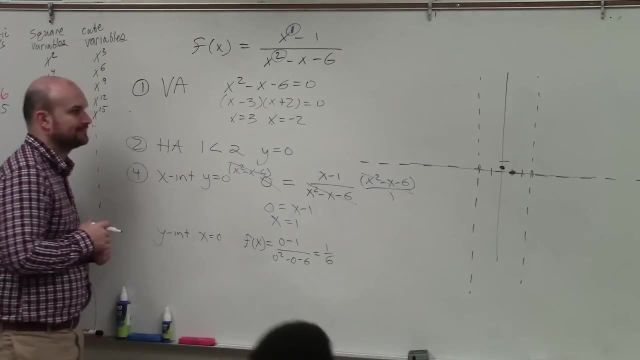 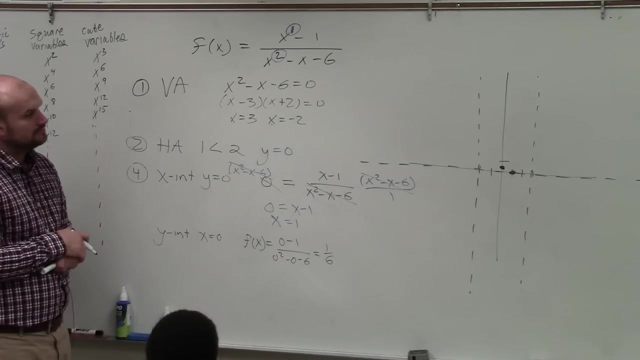 which equals 1 over 6.. So therefore, if this is 1,, 1, 6 is going to look something like that. OK, I have a question: Why are there y and x interceptions? Why are there x and y intercepts when this function doesn't even touch them? 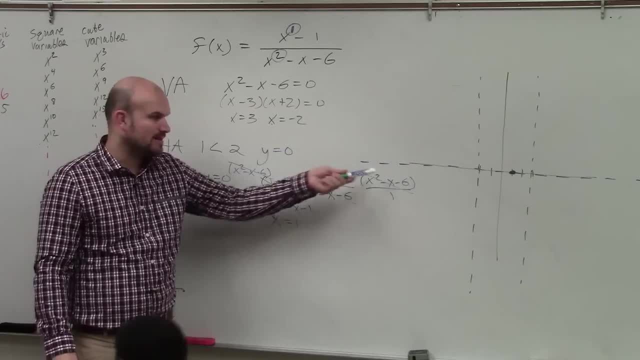 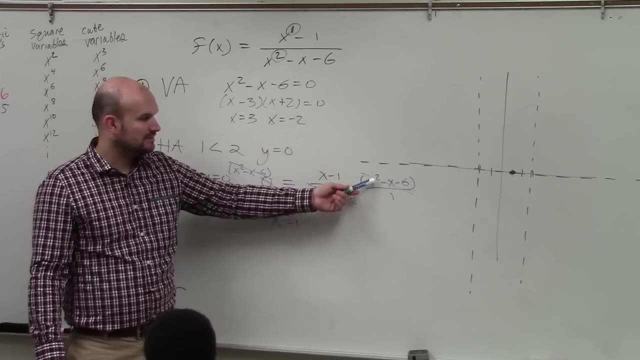 Well, I just want to get rid of what's in my denominator. So I multiply by the reciprocal of that. That eliminates what's in that denominator. That's the one I'm looking at, that denominator. right, if you multiply by the reciprocal, then you're still. 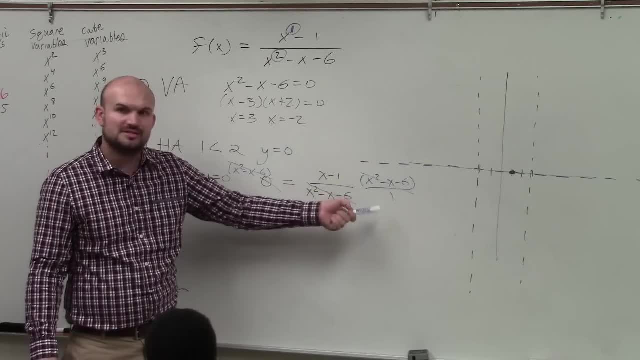 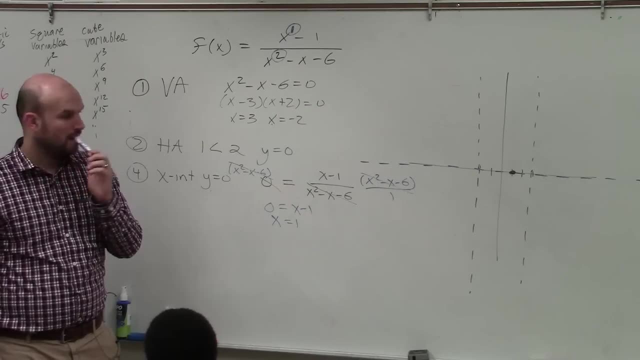 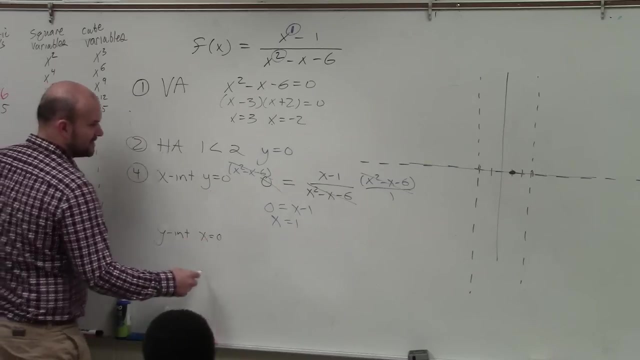 gonna have. then you have an X minus 1 in the denominator. you don't want to have any variables in the denominator, so I'm just multiplying by what's in the denominator. okay, so now the step. next one is to find the Y intercept. Y intercept X equals 0. so in this case I have f of X equals 0 minus 1, divided by 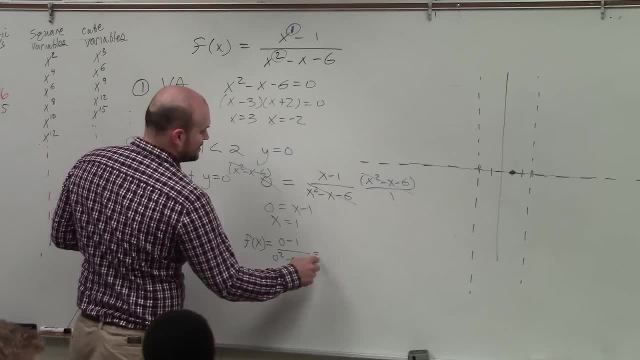 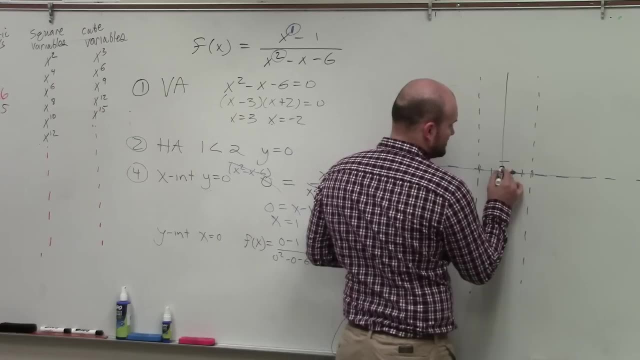 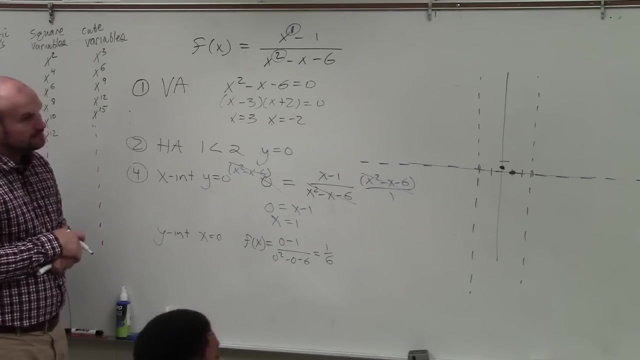 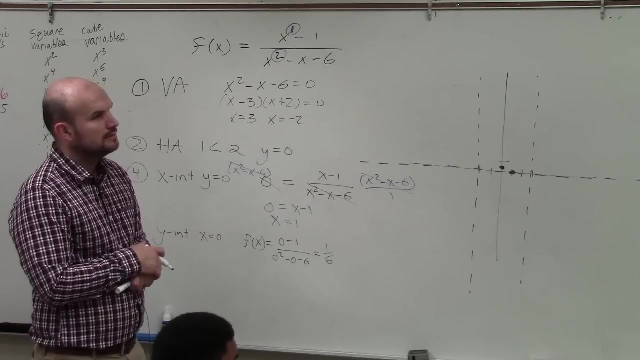 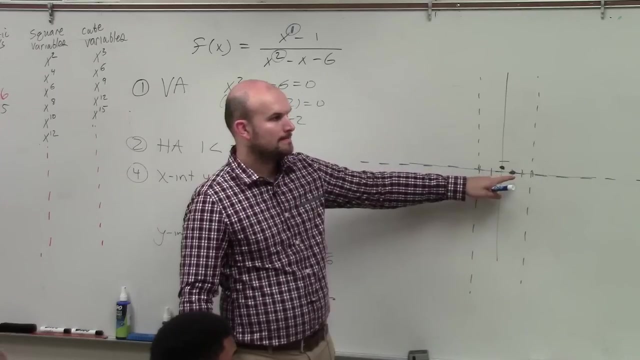 0 squared minus 0 minus 6, which equals 1 over 6. so therefore, if this is 1, 1, 6 is going to look something like that. okay, what it does? it touches them at 1- 6 and at 1 it does touch them. yes, you're correct. 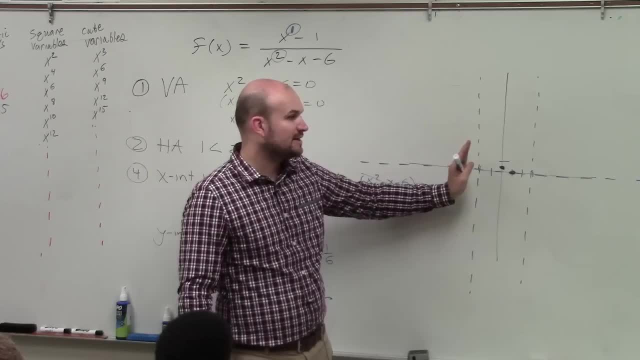 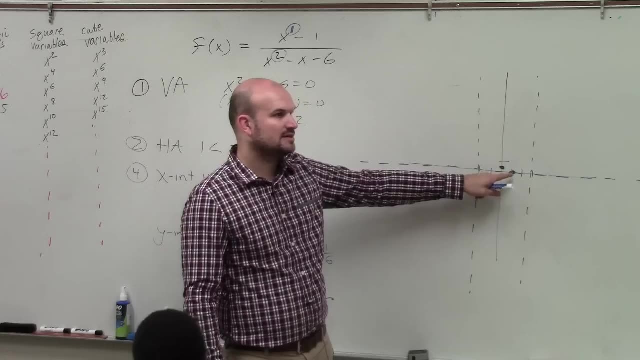 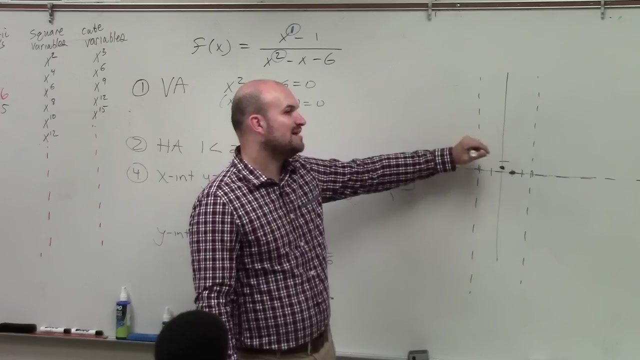 the vertical asymptotes are never going to be a part of them because these are rational functions. however, a horizontal asymptote you can actually cross, you can't have a value at a horizontal asymptote, because a horizontal asymptote is not going to be restricting your domain. however, for a 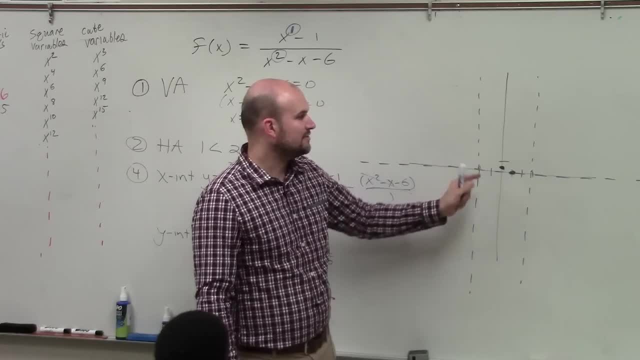 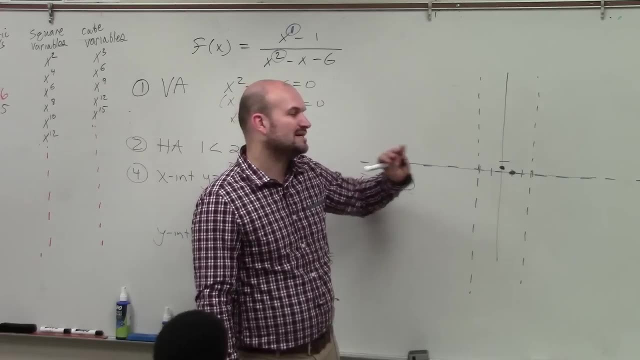 function. the vertical asymptotes restrict your domain. so therefore we can- will never- cross a vertical asymptote, but it is possible to cross that horizontal asymptote. I just want you to remember that the horizontal asymptotes, the main important thing to understand about asymptotes is that's going to be. 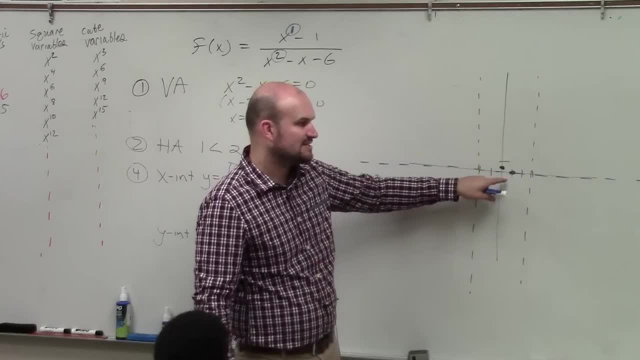 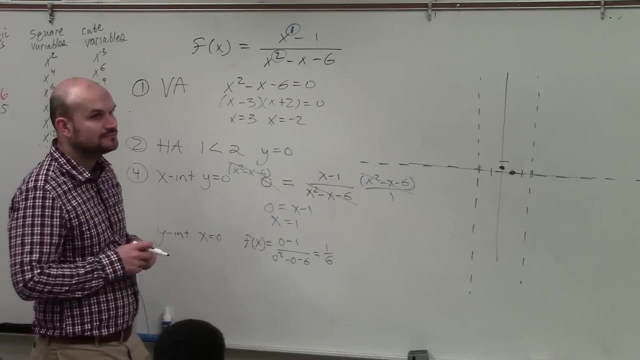 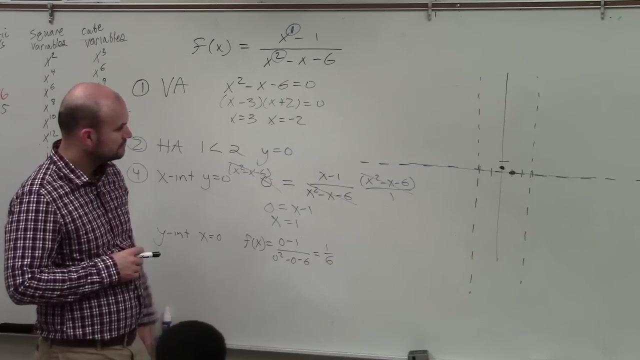 what your graph approaches. it's possible for it to cross this asymptote, but it's going to approach the asymptote and I'll explain that once we stick it to graphing. okay, yes, I did so. is the y wait? why is x equal to 1? 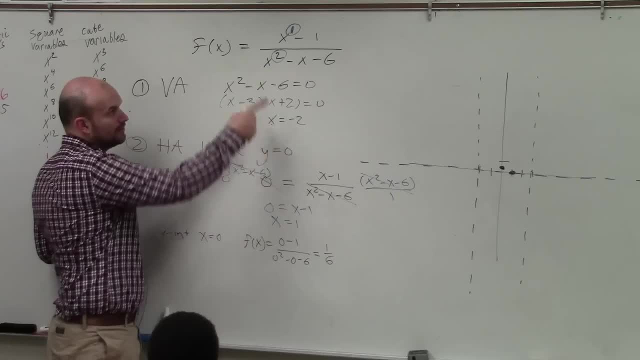 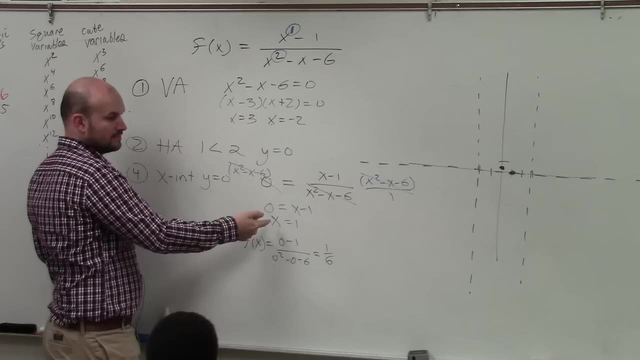 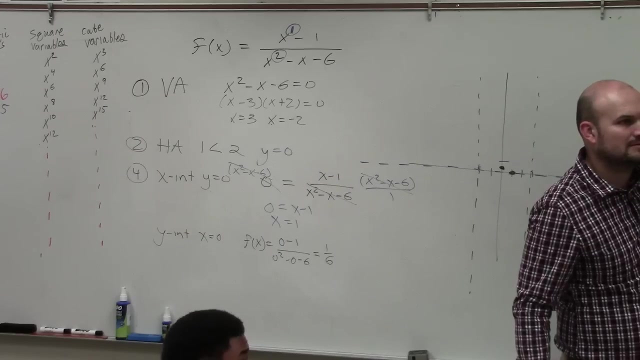 if you're changing the x equal to 0. I didn't. I replaced zero with y or, in reality, f of x. ah, so then that was find the x intercept. yep, you replaced f of x with y with x. yeah, because look at x intercept what is equal to zero, the y-coordinate right at y. 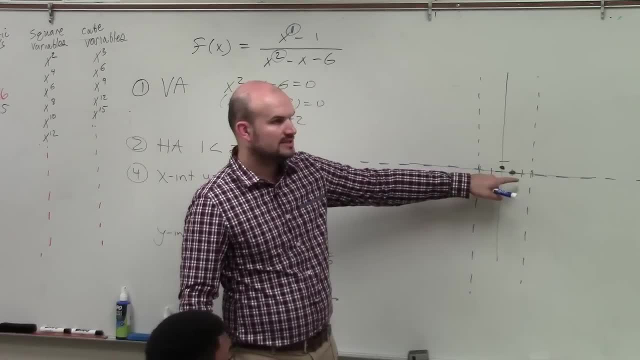 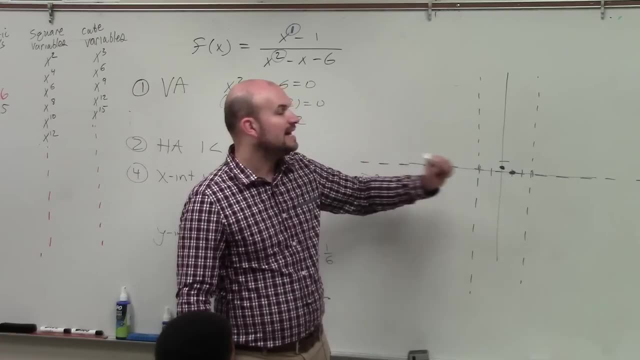 It does. It touches them at 1, 6 and at 1.. It does touch them. How? But it's not getting within the dot-dashed line. Yes, you're correct, The vertical asymptotes are never going to be a part of them. 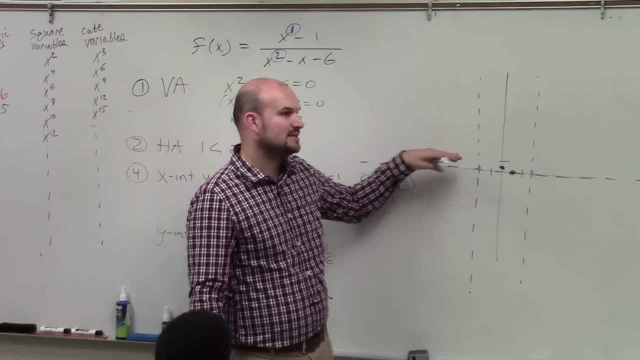 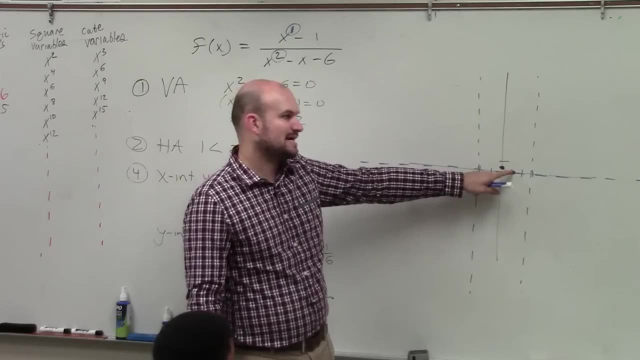 because these are rational functions. However, a horizontal asymptote you can actually cross, You can have a value at a horizontal asymptote, because a horizontal asymptote is not going to be restricting your domain. However, for a function, the vertical asymptotes- 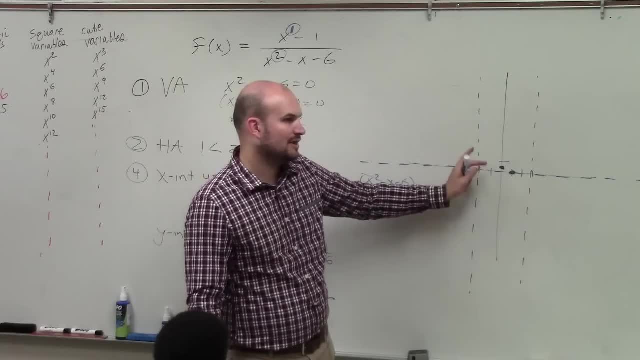 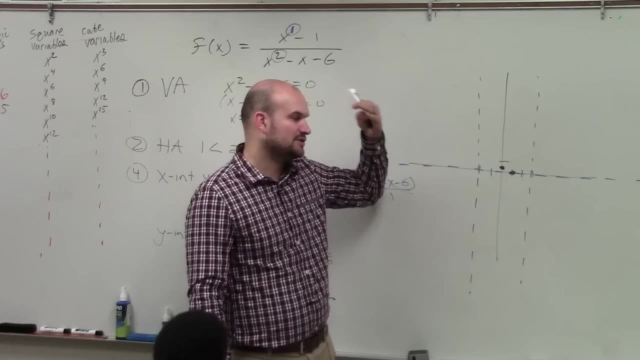 restrict your domain. So therefore, we will never cross a vertical asymptote, But it is possible to cross that horizontal asymptote. I just want you to remember that. the horizontal asymptotes, the main important thing to understand about asymptotes, is that's going to be what your graph approaches. 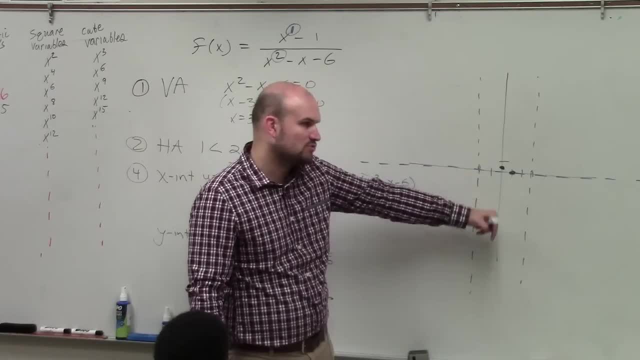 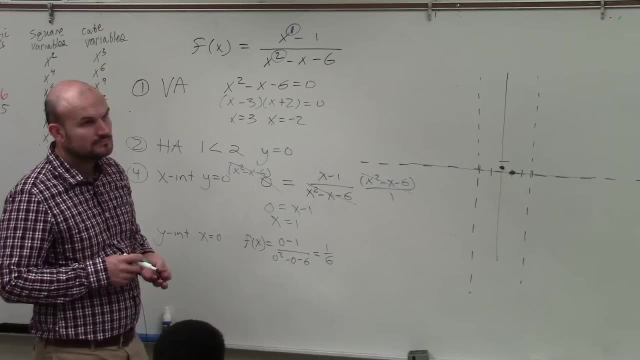 It's possible for it to cross this asymptote, but it's going to approach the asymptote And I'll explain that once we stick it to graphing. OK, Yes, Wait. So is the y? wait, why is x equal to 1? 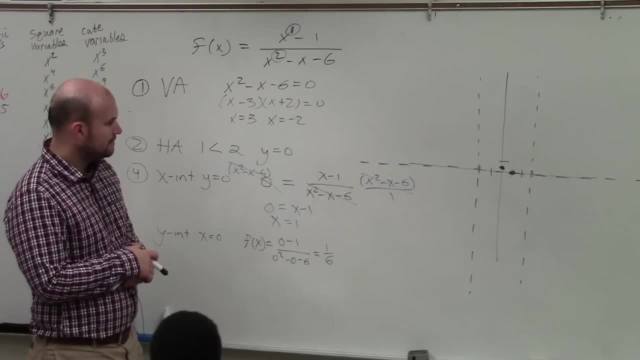 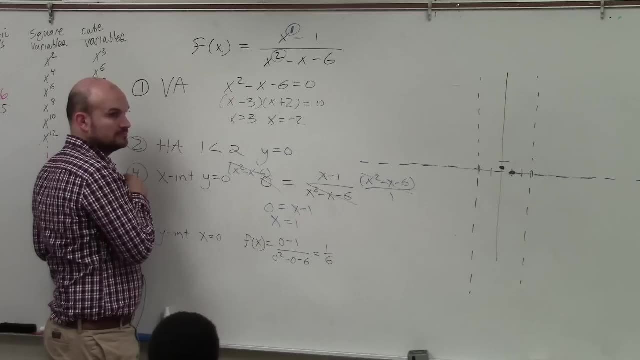 if you're changing the x equal to 0 and x equal to x. I didn't. I replaced 0 with y or, in reality, f of x. Yeah, so then that would find the x and the z. Yep, So you replace the 0 with x. 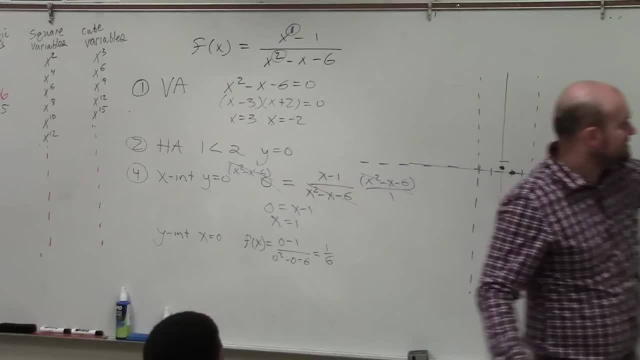 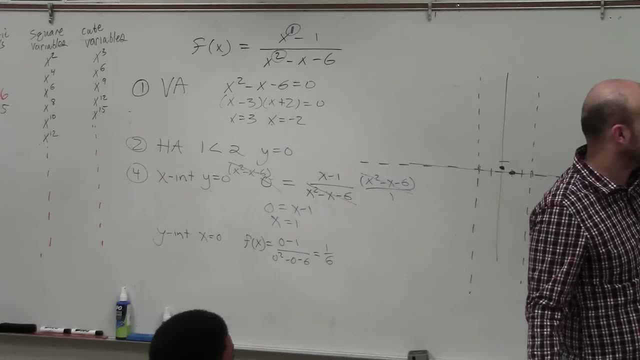 Yeah, because look it. x-intercept, what is equal to 0? The y-coordinate Right At y-intercept, what's equal to 0? The x-coordinate Right. So when I said, hey, I want to find the y-intercept. 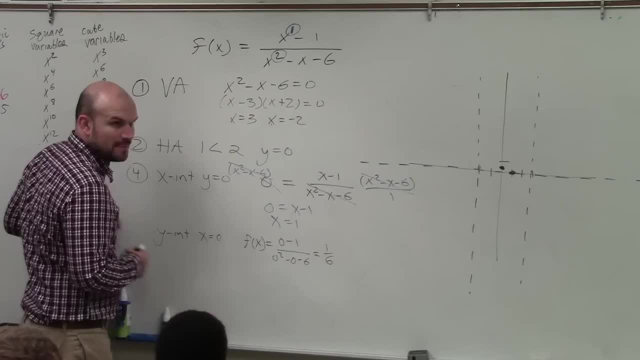 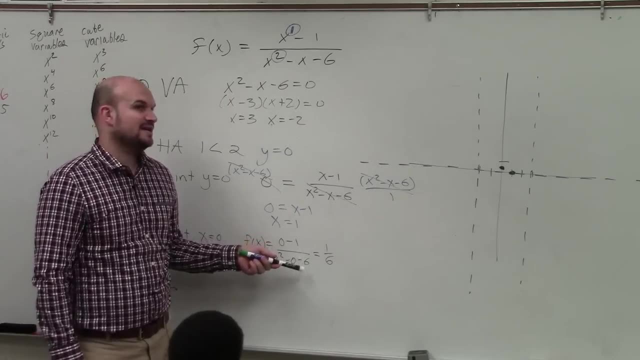 x equals 0. So I plug 0 in for x. Make sense, OK? Yes, Is it 1 over 6, or is it negative? It's negative 1 over negative 6,, which reduces to 1 over 6.. 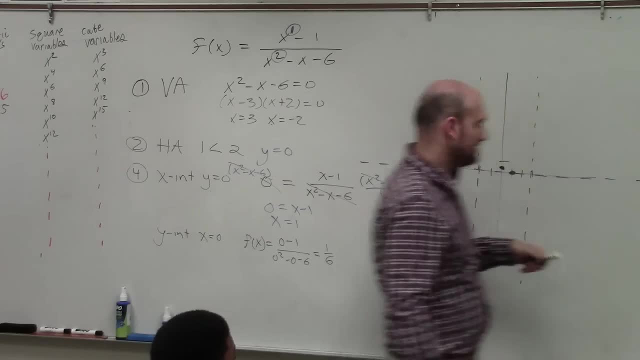 intercept what's equal to 0. What's equal to 0? The x-coordinate. So when I said, hey, I want to find the y-intercept, x equals 0. So I plug 0 in for x, Make sense. 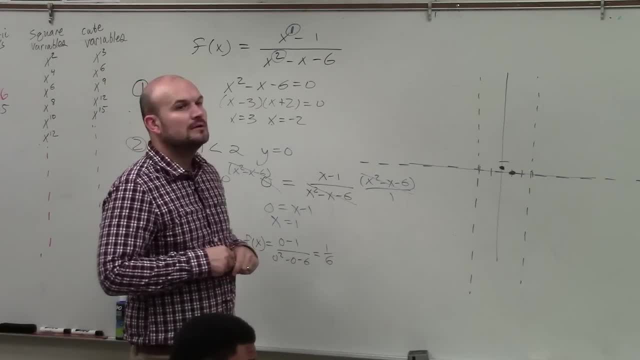 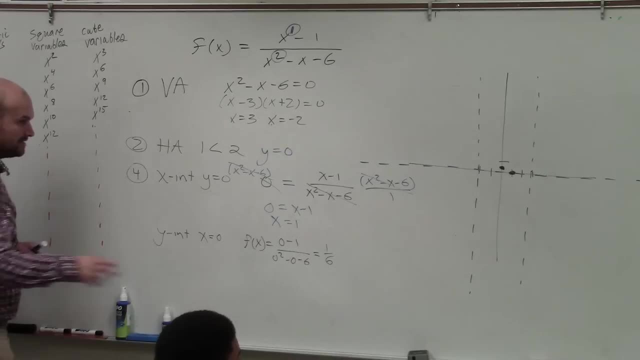 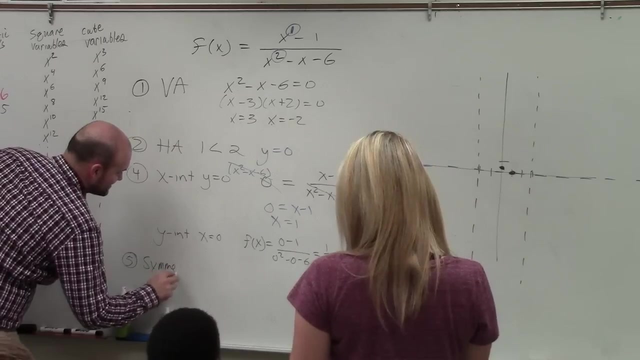 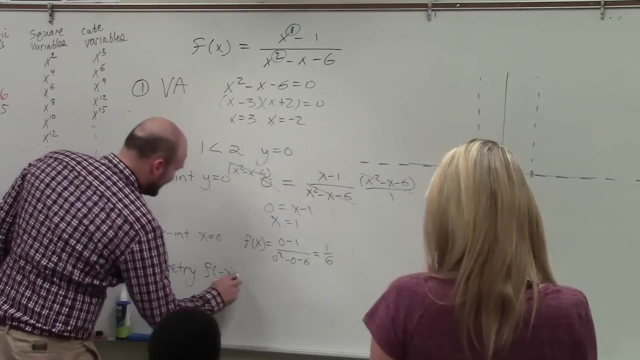 OK, Yes, Is it 1 over 6, or is it negative 1?? It's negative 1 over negative 6, which reduces to 1 over 6.. The next thing is for us to text symmetry, which we're going to do: f of negative x equals negative x minus 1. 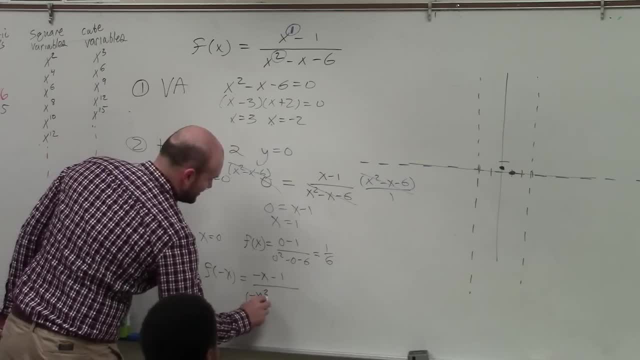 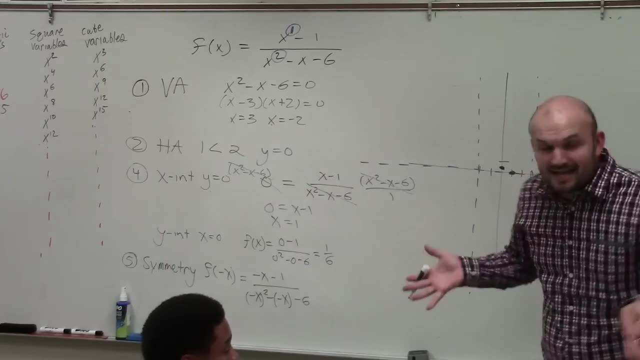 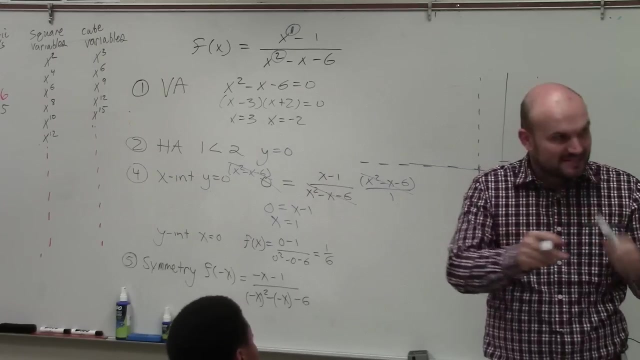 all over: negative x squared minus negative x minus 6.. Now, when you go ahead and simplify this, if you get the exact same answer, you have symmetry about the y-axis, right, If you get the exact same answer, but with opposite signs. 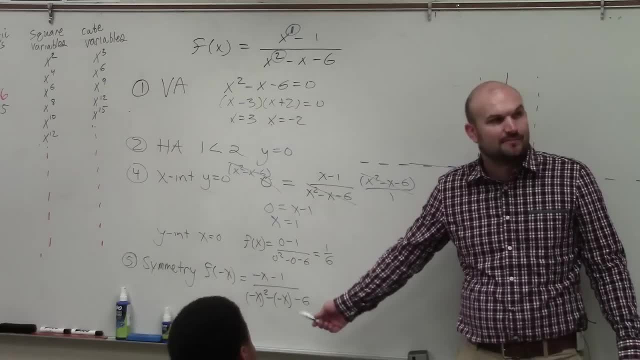 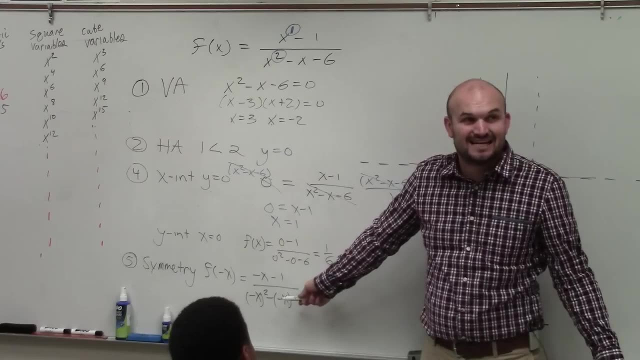 you have symmetry about the origin. Well, I'm not going to spend time simplifying this, because I already know that my numerator is not the exact same as my numerator over here, and it's not the exact opposite either: Negative- positive. 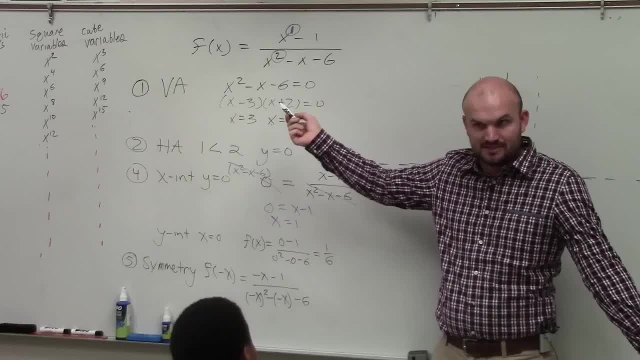 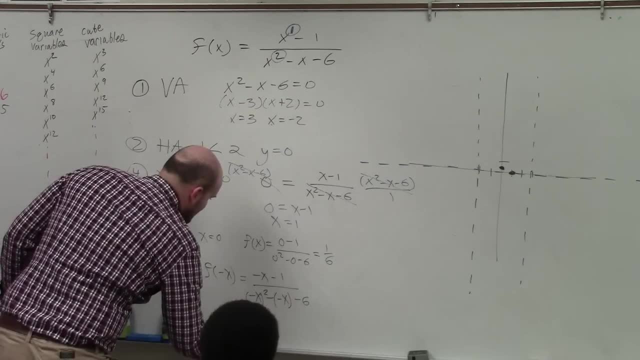 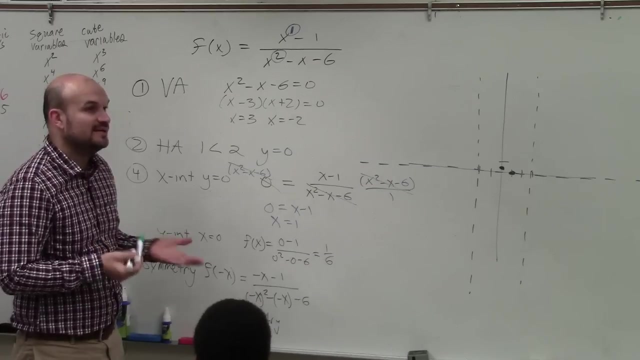 Those are opposites, but then that's negative, negative, which doesn't work. Does that make sense? Yes, So there's no symmetry, So you can just write no symmetry. Now the last thing we need to do is plot points. 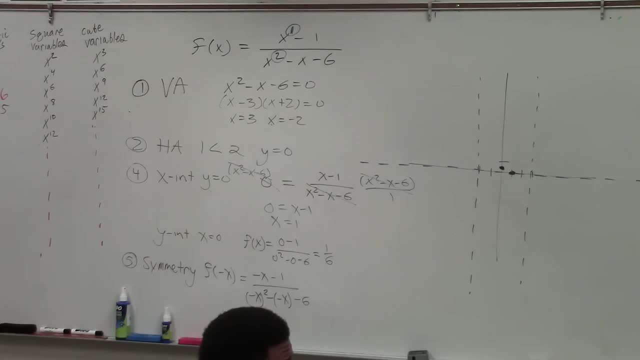 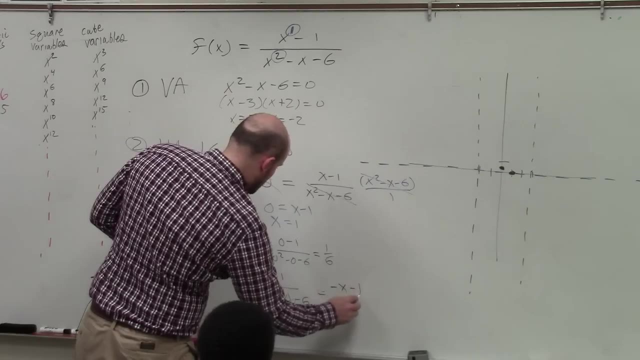 Yes, So is there a symmetry? when you plug all your x's and negatives, Yeah, you're basically evaluating for f of negative x, And now, in reality, you've got to simplify this, which, since you're having a question, I'll simplify it. 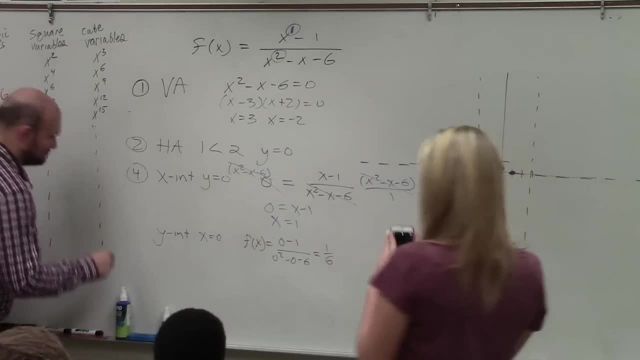 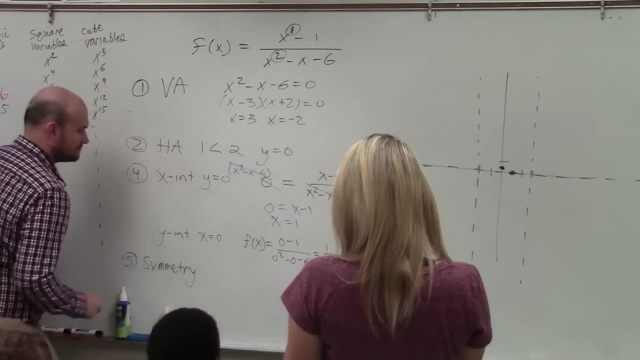 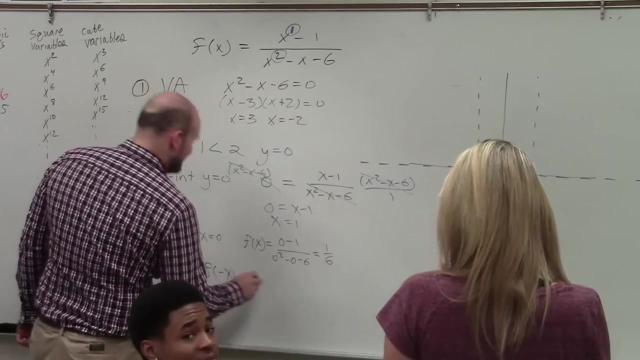 How difficult is that really? Yeah, just wait a minute, OK. The next thing is for us to text symmetry, which we're going to do: f of negative x, f of negative x equals negative x minus 1, all over negative x. 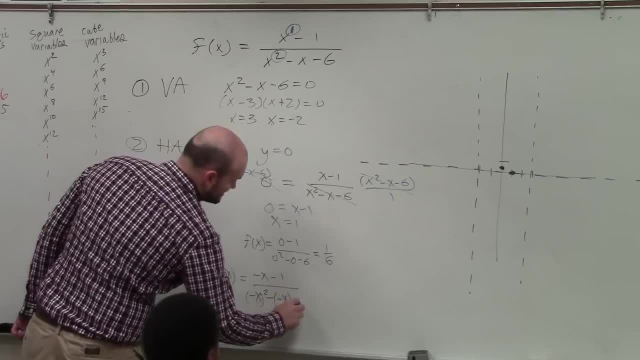 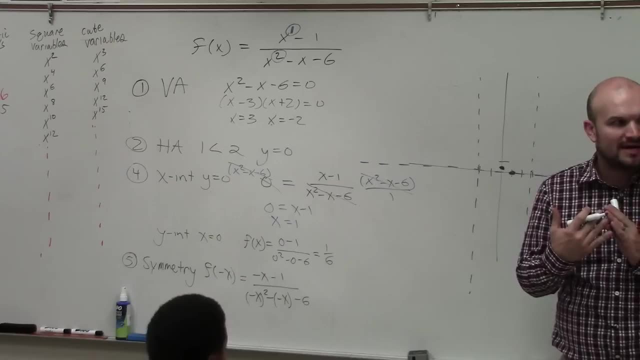 squared minus negative, x, minus 6.. Now, when you go ahead and simplify this, if you get the exact same answer, you have symmetry about the y-axis, Right. If you get the exact same answer, but with opposite signs, you have symmetry about the origin. 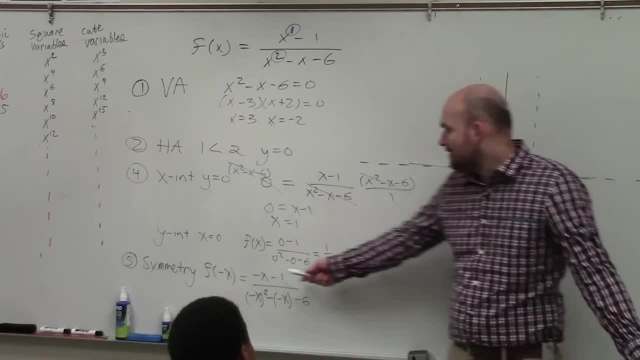 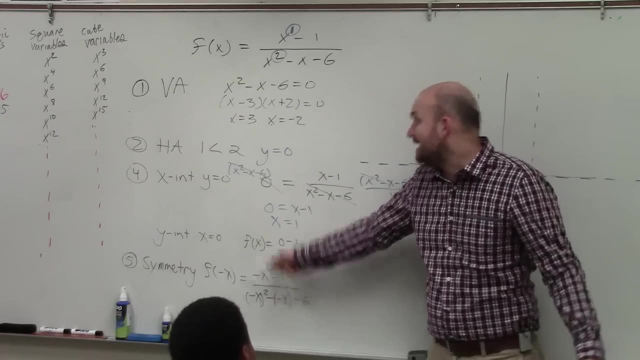 Well, I'm not going to spend time simplifying this, because I already know that my numerator is not the exact same as my numerator over here, and it's not the exact opposite either. Negative, positive, Those are opposites, but then that's negative, negative. 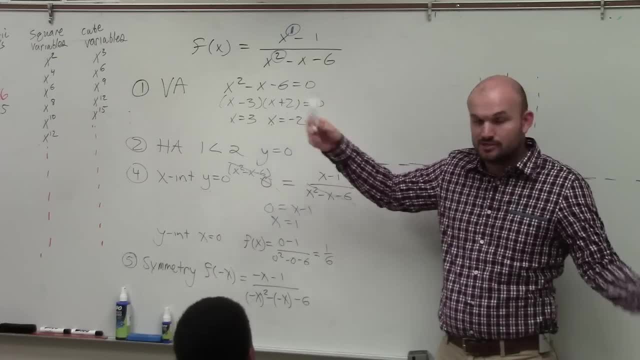 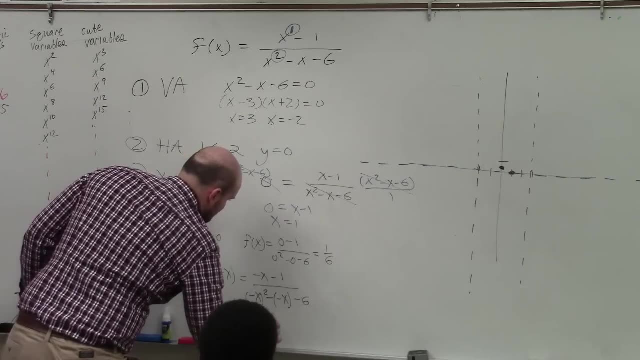 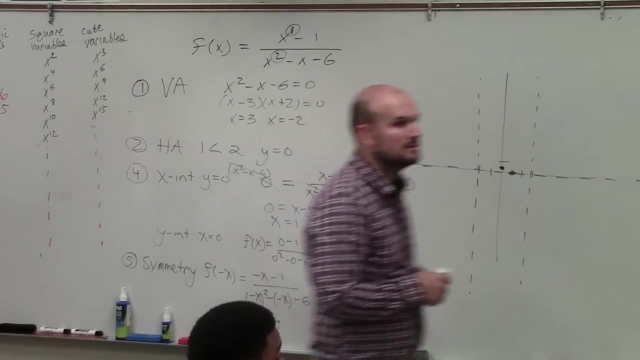 which doesn't work. Does that make sense? Yes, So there's no symmetry. So you can just write: no symmetry, Symmetry. OK, Now the last thing we need to do is plot points. Yes, So for the symmetry you use all your x's and negatives. 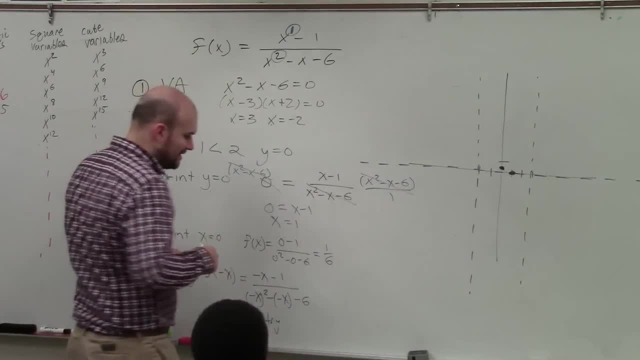 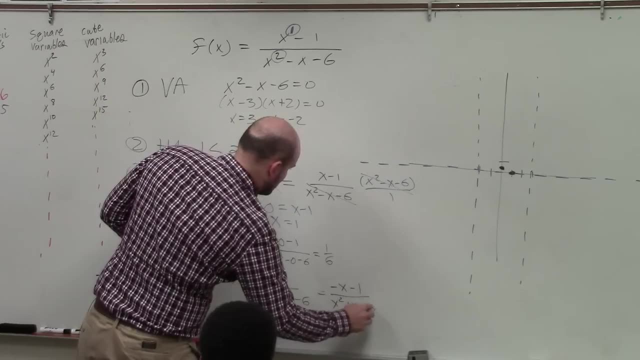 Yeah, You're basically evaluating for f of negative x, And now, in reality, you've got to simplify this, Which, since you're having a question, I'll simplify it. You will. There's the examples. I don't know if we'll do one today. 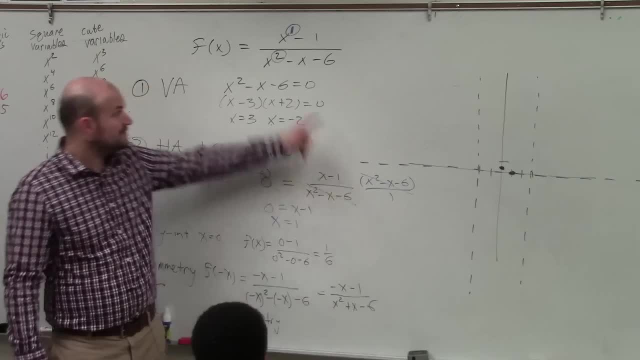 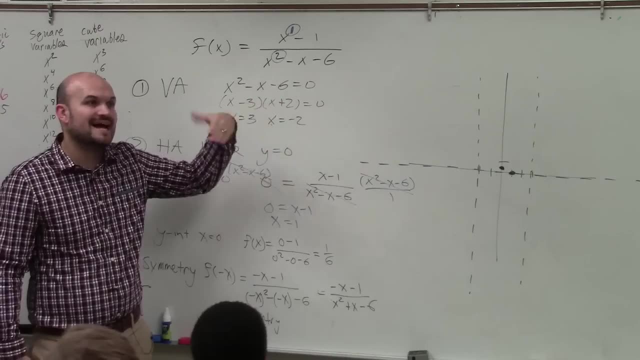 But So here, when I plug in negative x and simplify, do I have the exact same function? No, Do I have the exact same function, but with everything being the opposite sign No, No, So there's no symmetry, It's not even. 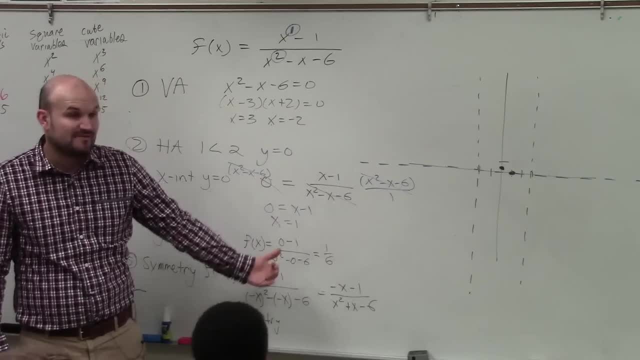 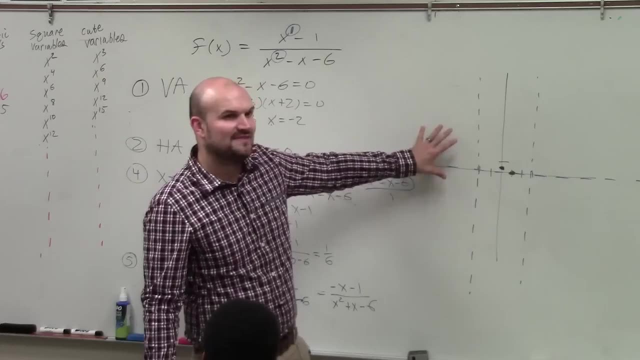 This is nor an even nor an odd function. OK, However, there will be examples when you have even or odd. And what's nice about them, especially if you have even? if you have even, you can just graph on the left side. 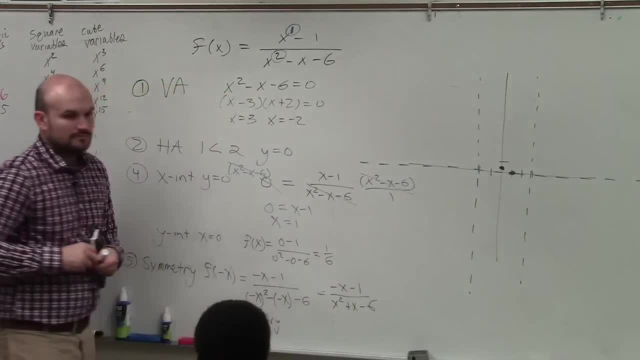 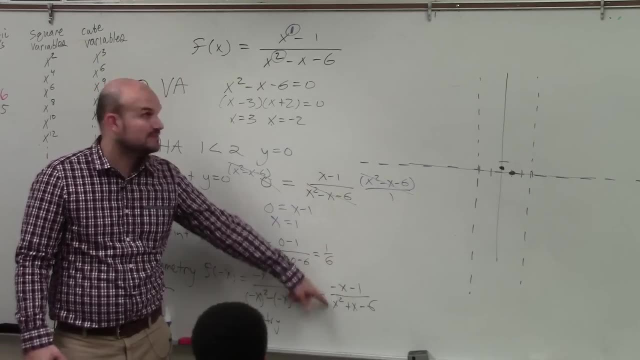 There's one where it's going to be the same as You will. There's the examples. I don't know if we'll do one today. So here, when I plug in negative x and simplify, do I have the exact same function? 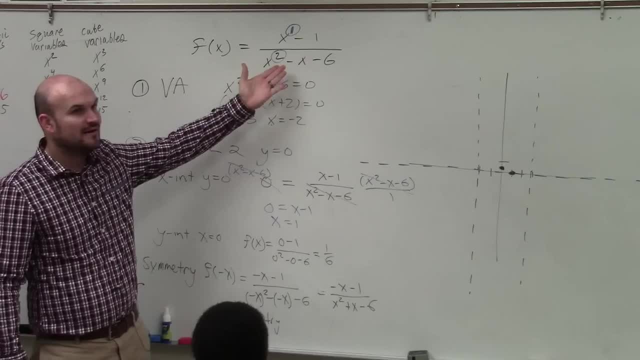 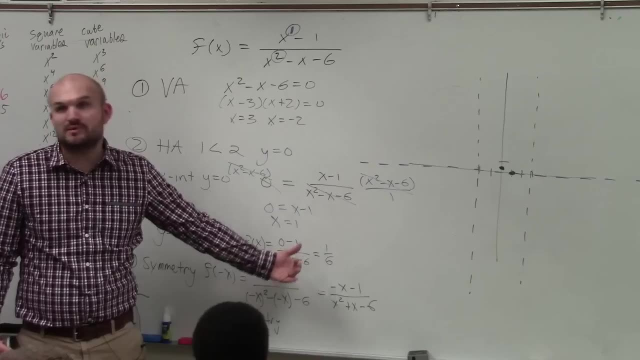 No, No. Do I have the exact same function, but with everything being the opposite sign? No, No. So there's no symmetry. It's not even. This is nor an even nor an odd function. However, there will be examples when you have even or odd. 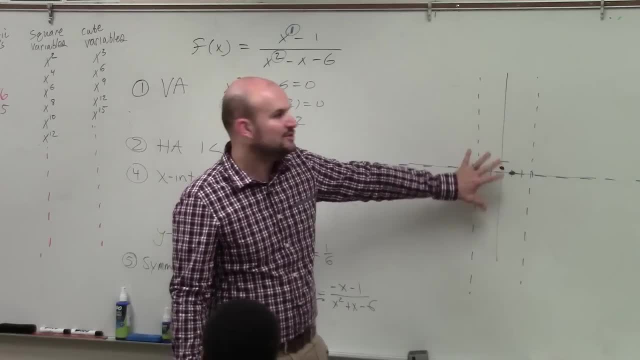 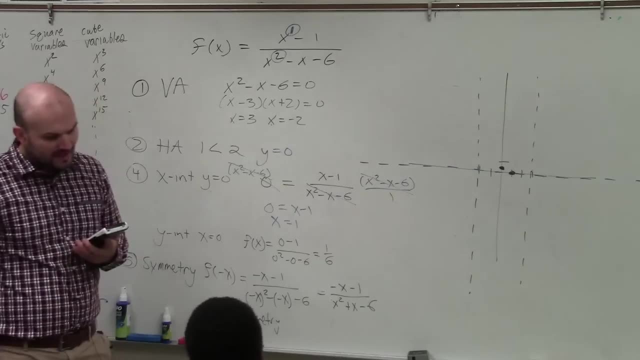 And what's nice about them, especially if you have even. if you have even, you can just graph on the left side and then flip it over, And that's what's nice about even functions. Now the table: Basically, as we've done with the table of values, 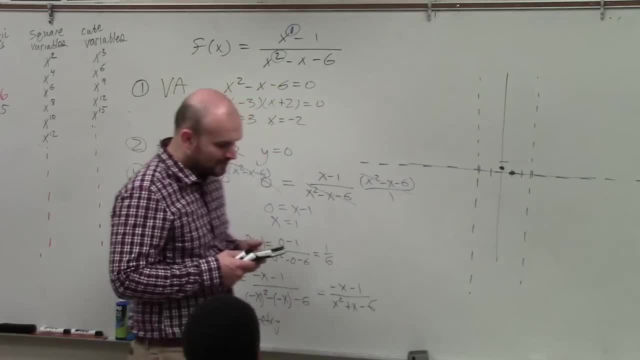 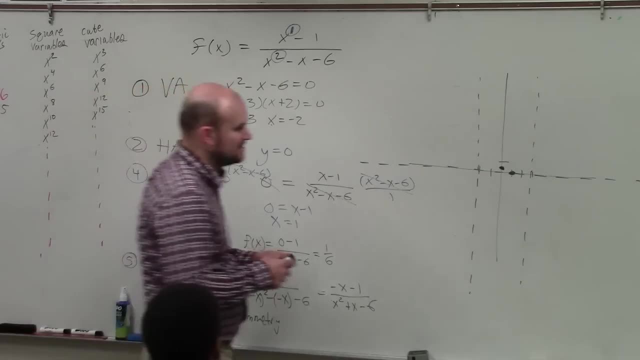 and then flip it over Right, And that's what's nice about even functions. Now the table: All right, Basically, as we've done when the table of values- you're going to have a table of values, You're going to want to pick some points. 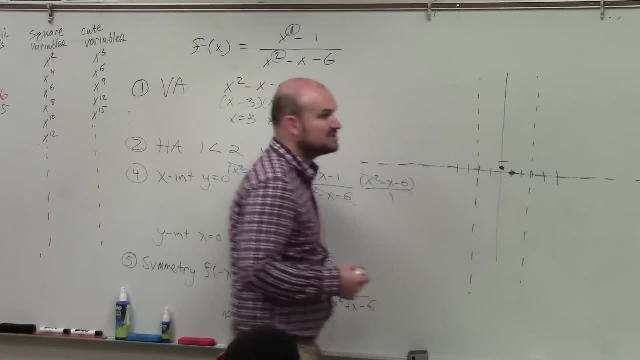 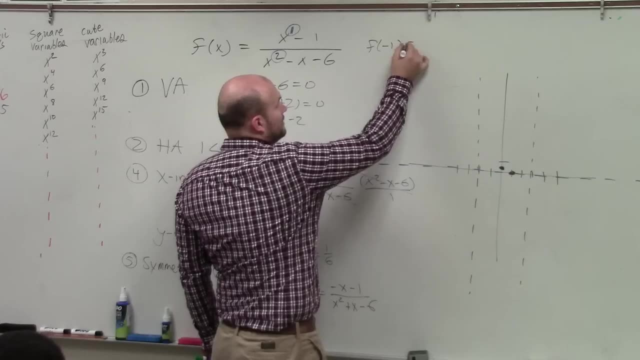 For those of you that don't have a calculator, you need to know what this graph looks like, Right? So you need to evaluate this function. for some other points, I would maybe evaluate for negative 1.. I would maybe evaluate for 1,, 2, 3.. 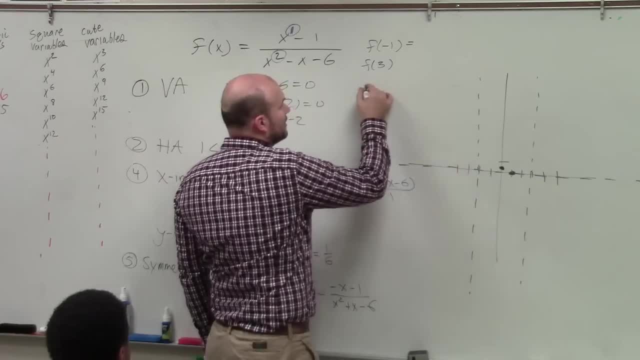 Plug in f of 3.. Plug in f of 1,, 2,, 3, 4.. Plug in 1,, 2,, 3,, 4, 5.. Oh, that's negative 4 and negative 3.. 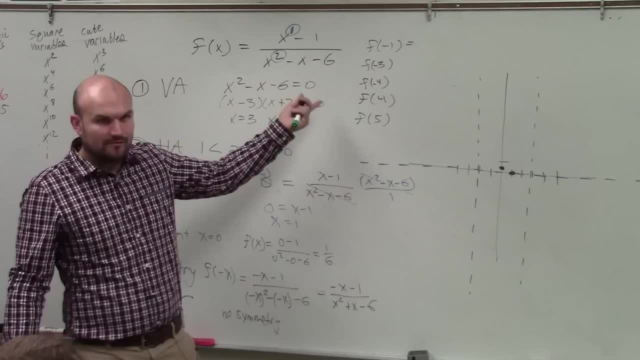 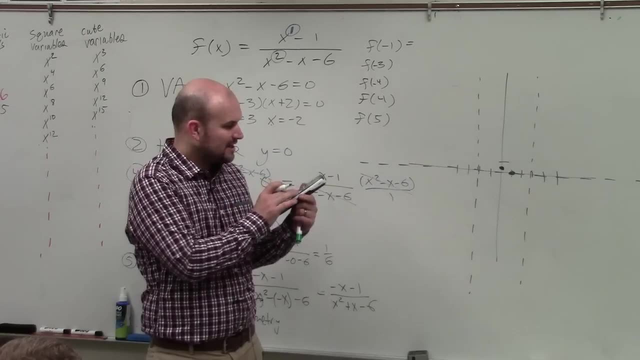 And you plug those numbers in for x and then find what f of x is Right And then you plot them. If you have a calculator, or at least access to a calculator, you can type in your calculator and just go to the table function. 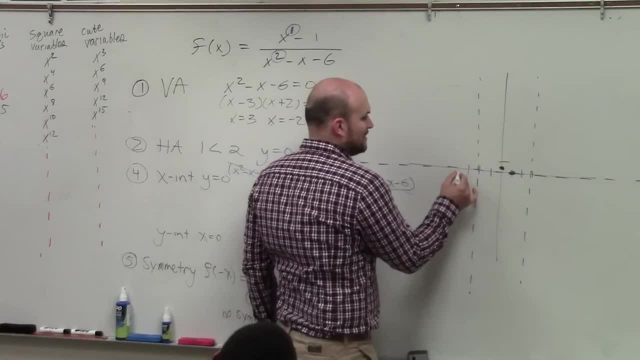 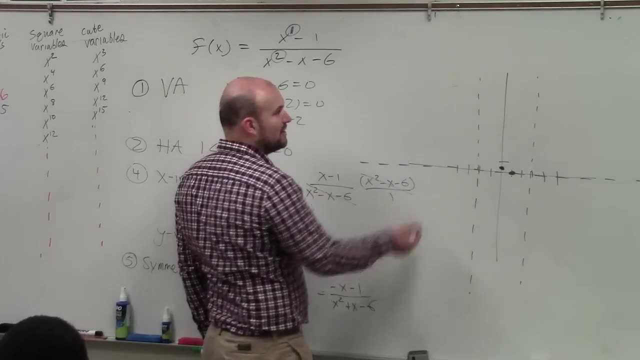 you're going to want to pick some points. For those of you that don't have a calculator, you need to know what this graph looks like, So you need to evaluate this function. for some other points, I would maybe evaluate for negative 1.. 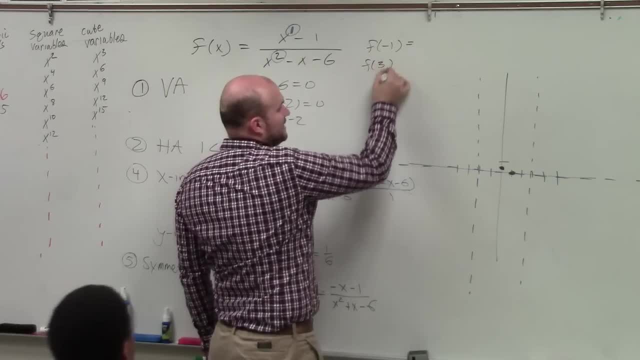 I would maybe evaluate for 1,, 2,, 3. Plug in f of 3. Plug in f of 1,, 2,, 3, 4. Plug in 1,, 2,, 3,, 4, 5.. 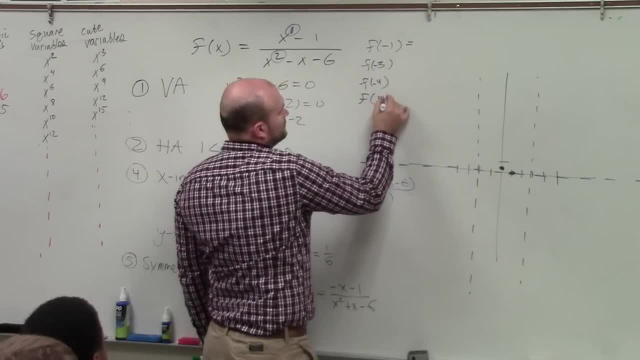 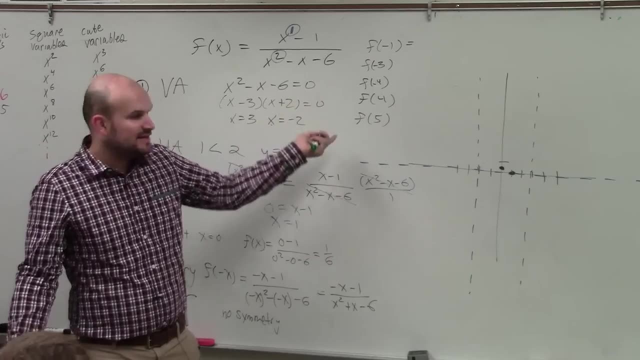 Oh, that's negative 4 and negative 3. And you plug those numbers in for x and then find what f of x is right And then you plot them If you have a calculator, or at least access to a calculator, 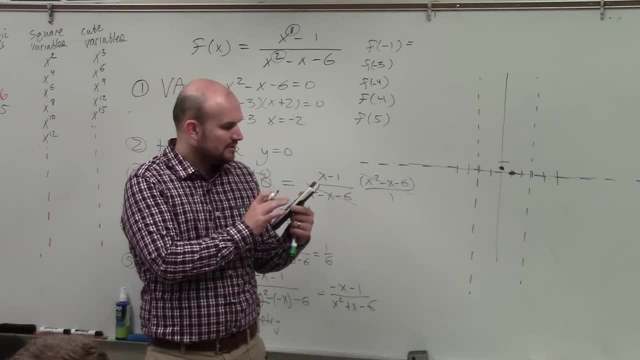 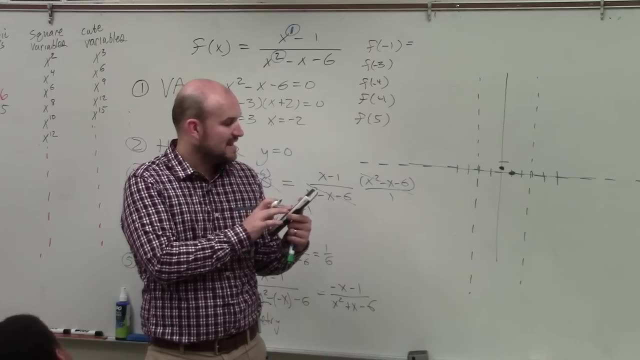 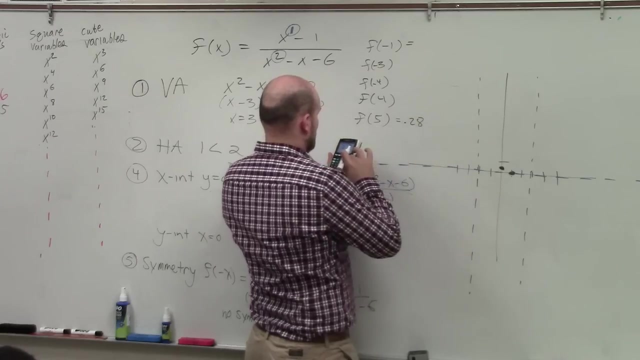 you can type in your calculator and just go to the table function, And then that will actually tell you what they are without having to do all that algebra. And so, for the sake of time, f of 5 is 0.28.. f of 4 is 0.5.. 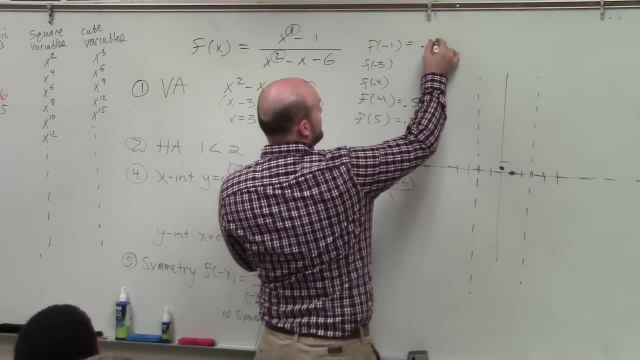 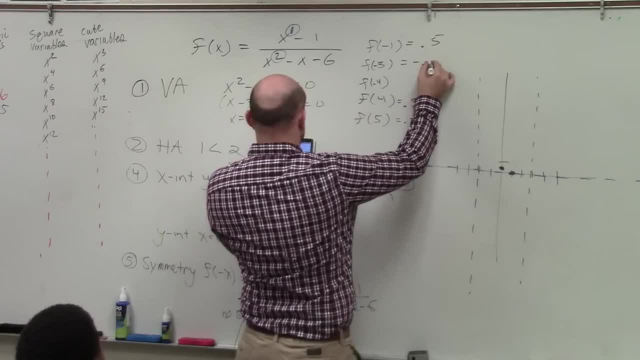 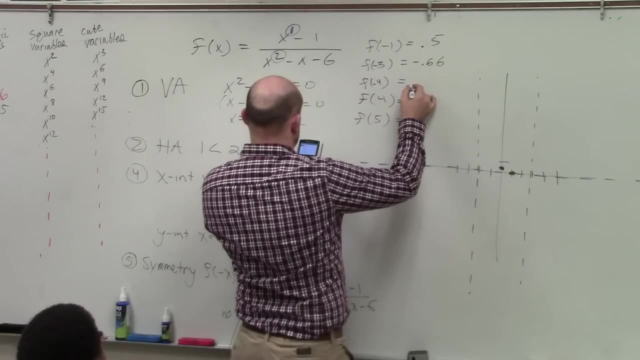 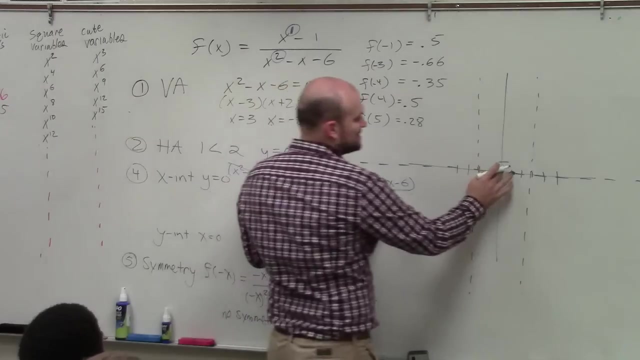 0.5.. That's negative 2.66.. And f of negative 0.66.. So this is just a little bit of example. But remember, this was like 1,, 6, right? So I was really like there. 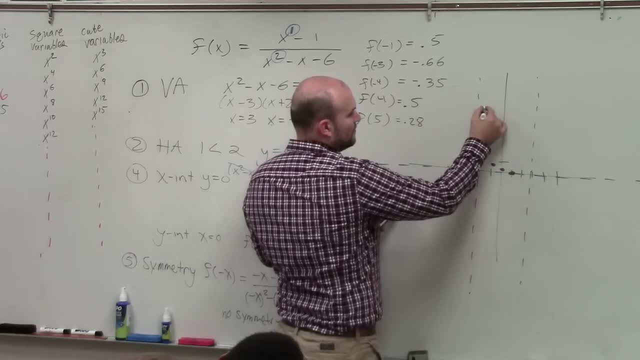 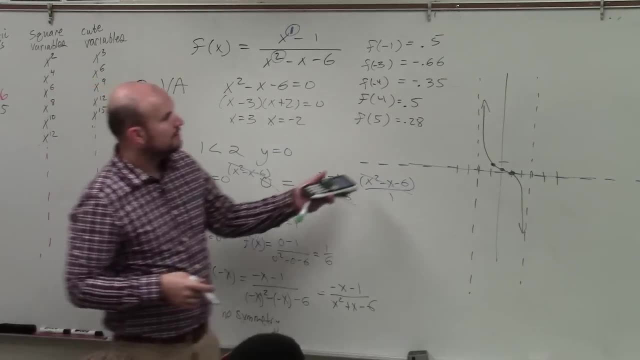 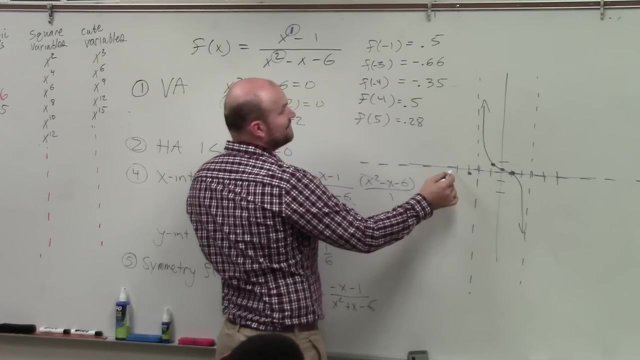 And negative 1, I'm at 0.5.. So what this graph is doing is creating something like this: OK, Over here at negative 4, that's at 0.5.. But then at negative 5, it's at or at negative. I'm sorry. 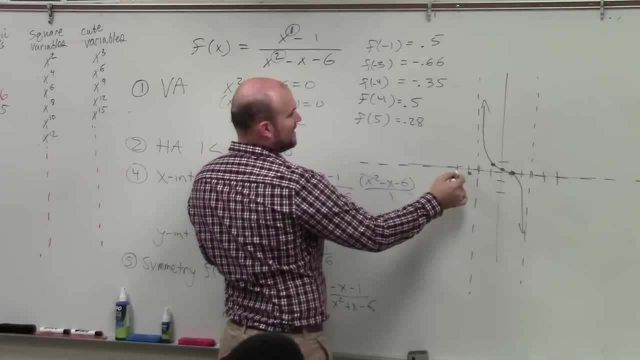 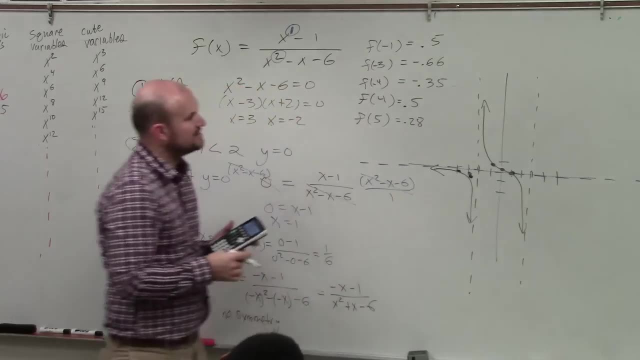 at negative 4, it's at 0.35.. And here it's at 0.66.. What that graph is doing is doing that, And then at 4 and 5, at 4, 1,, 2,, 3, 4, I'm at 0.5.. 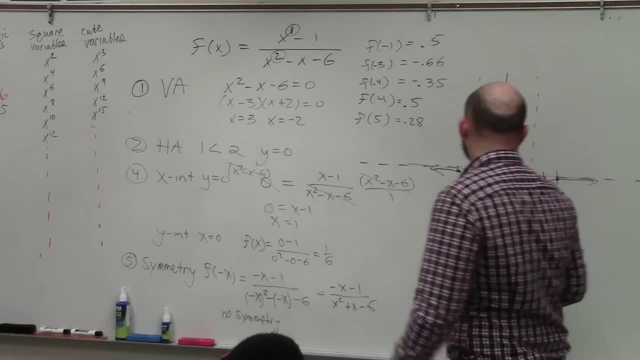 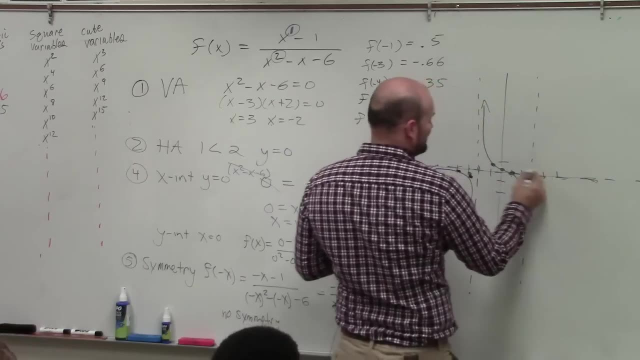 And then at 0.25. 0.25., 0.25. 0.25.. That's wrong, That's totally wrong. Oh no, I'm sorry, That's positive, not negative. Thank you, You're right. 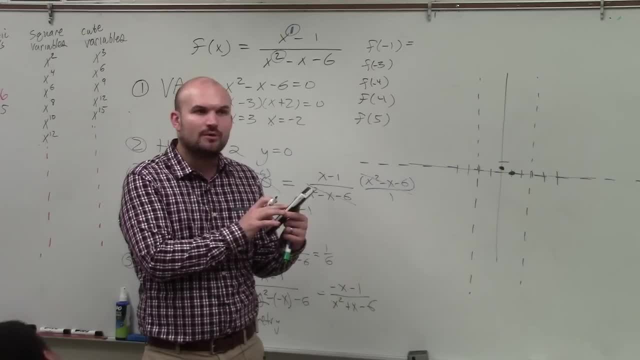 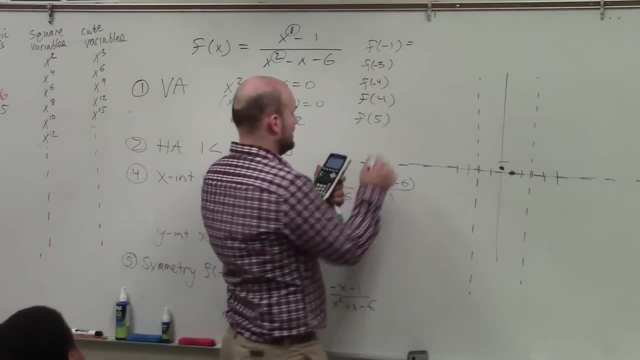 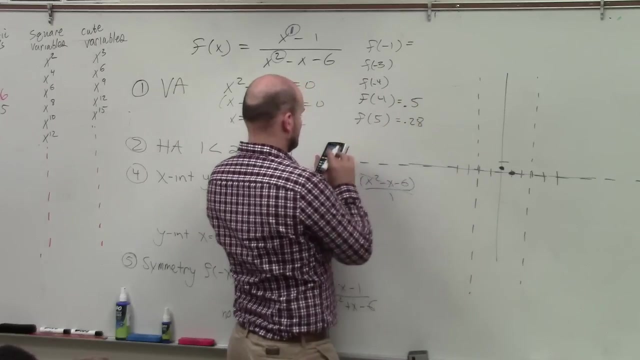 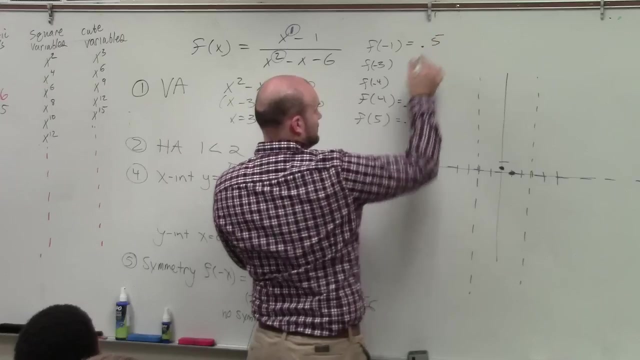 And then that will actually tell you what they are without having to do all that algebra. And so, for the sake of time, f of 5 is 0.28.. f of 4 is 0.5.. f of negative 1 is 0.5.. 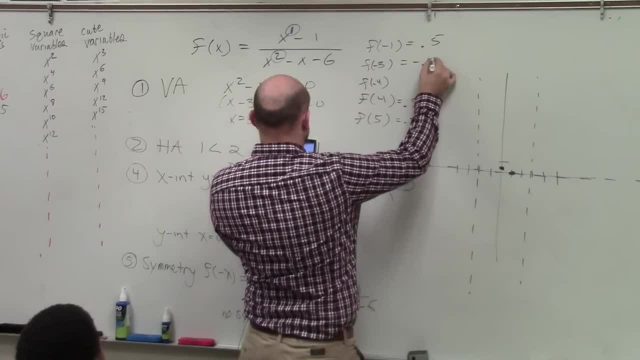 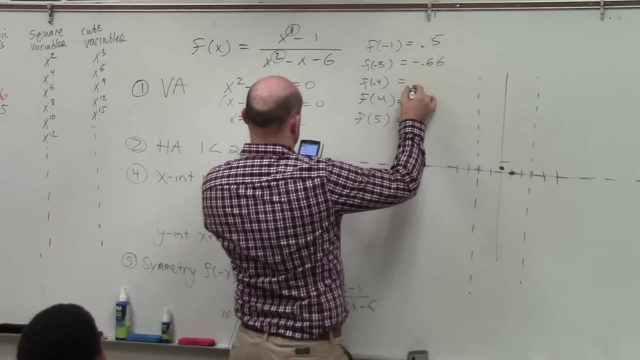 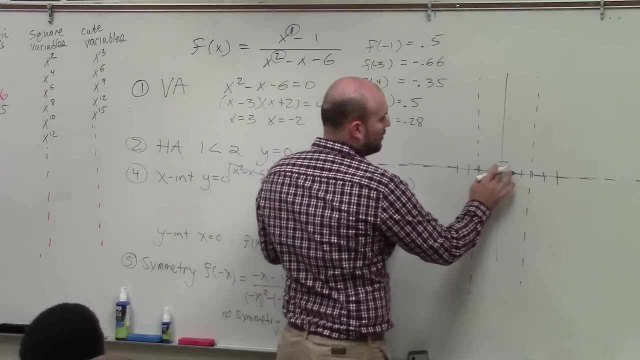 That's negative 2.66.. And f of negative 0.66.. So this is just a little bit of example, But remember this was like 1, 6.. Right, So it was really like there At negative 1, I'm at 0.5.. 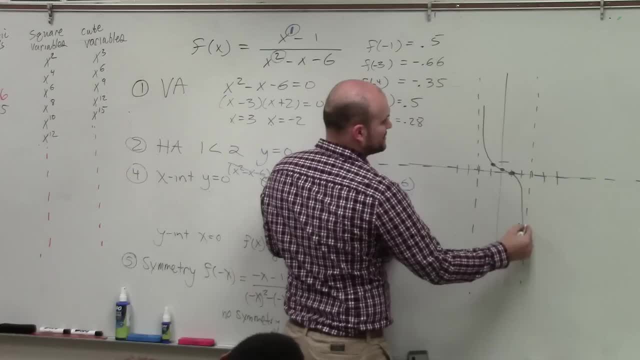 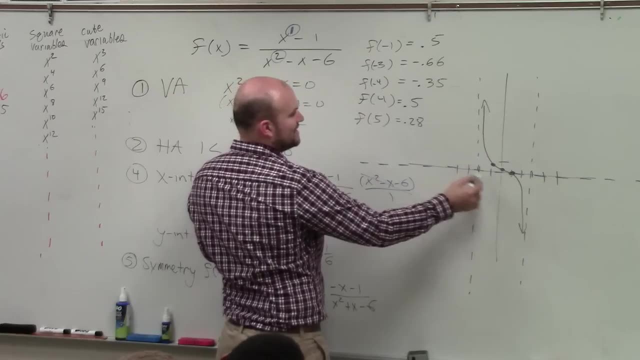 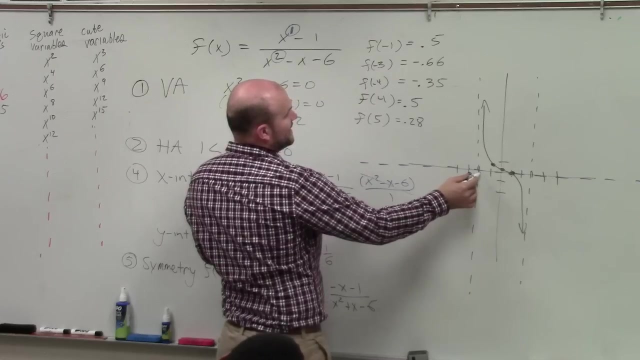 So what this graph is doing is creating something like this: OK, Over here, at negative 4, that's at 0.5.. But then at negative 5, it's at, or at negative, I'm sorry, at negative 4, it's at 0.35.. 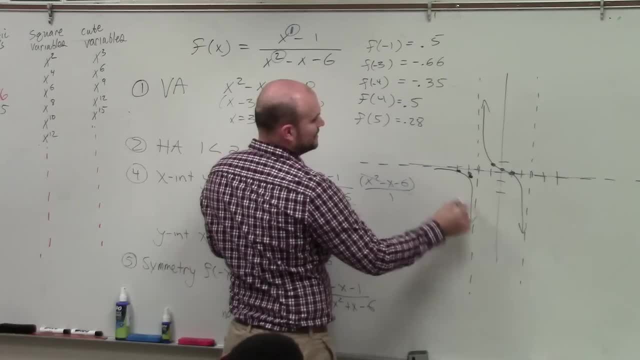 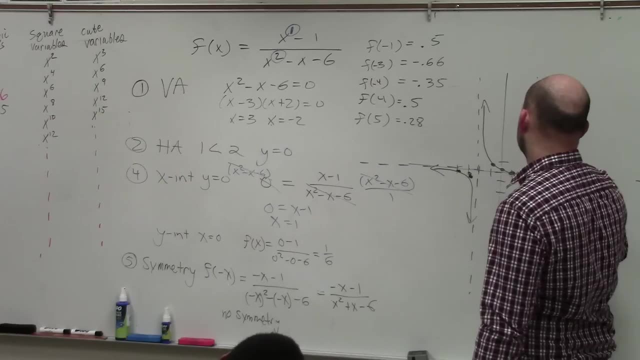 And here it's at 0.66.. What that graph is doing is it's just doing that, And then at 4 and 5, at 4, 1,, 2,, 3, 4, I'm at 0.5.. 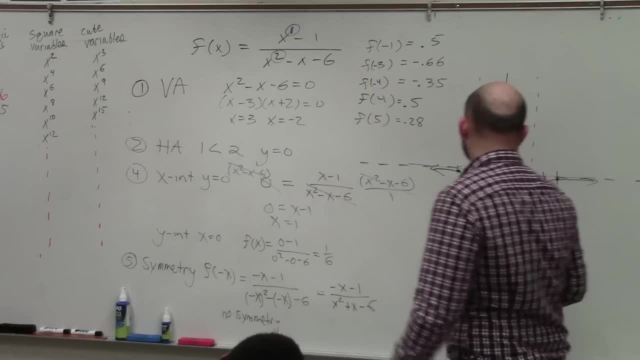 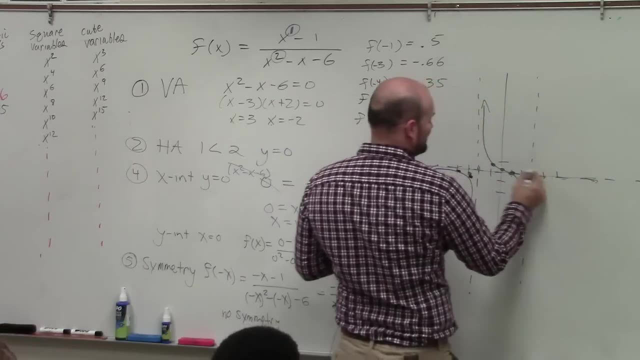 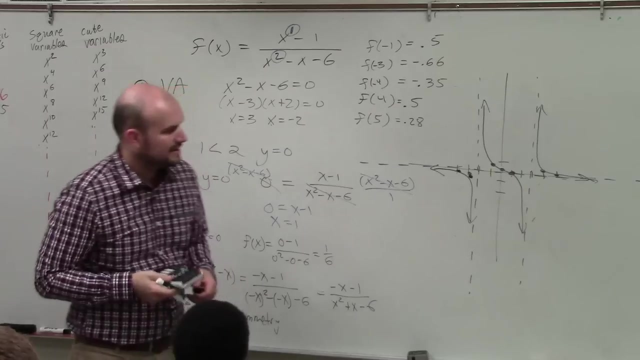 And then at 0.25.. That's wrong, That's totally wrong. Oh no, I'm sorry, That's positive, not negative. Thank you, You're right, Those are positive, Positive and positive. OK, I'll show you exactly what I think. 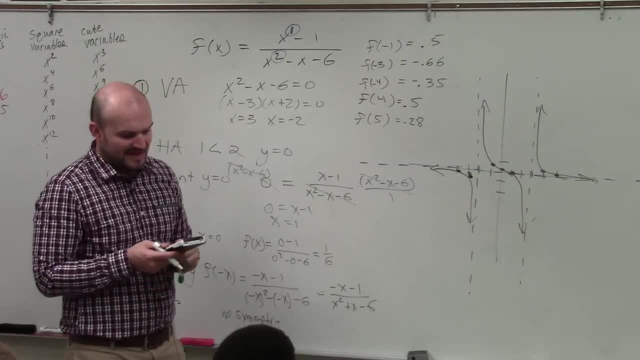 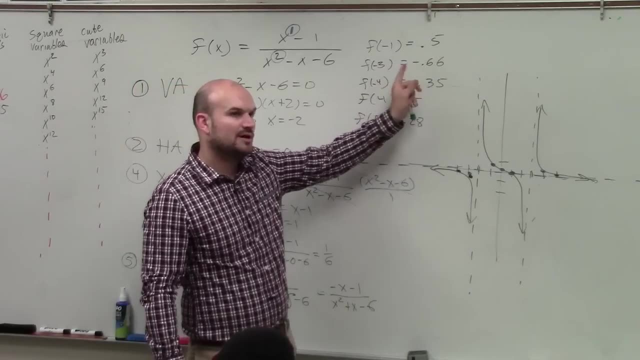 But yeah, those are positive values, Those are the negative right. So that's what, technically, your graph would be able to look at. All I'm asking you guys to do is basically being able to. Obviously, you're going to want to plug in some points. 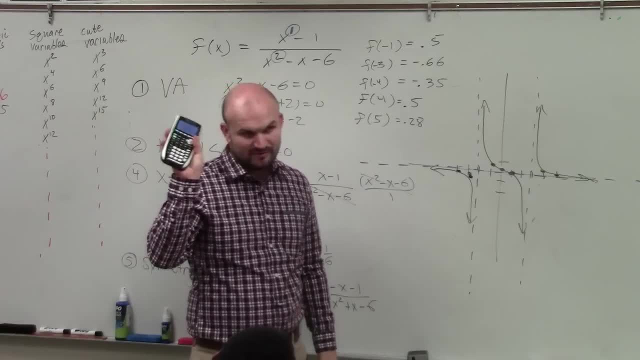 enough that you know what the graph shape is going to look like, But having a graph calculator would be very, very helpful for you. OK, Zach, are you OK?